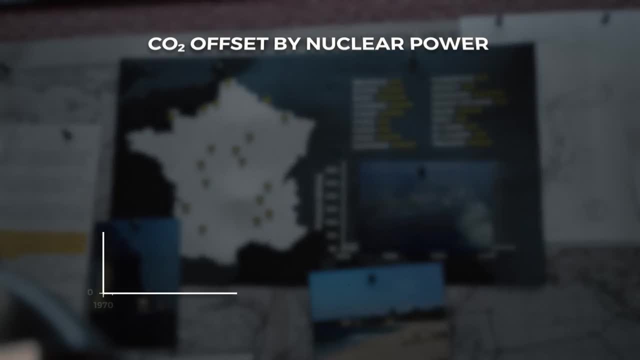 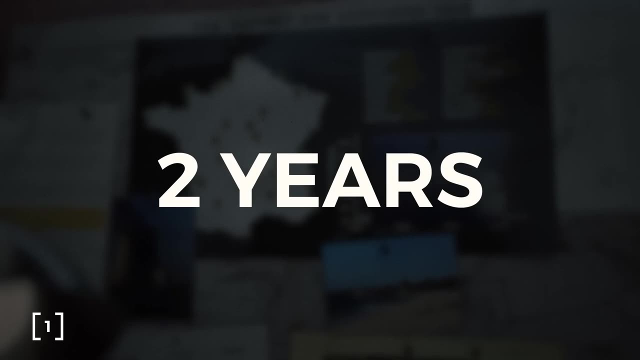 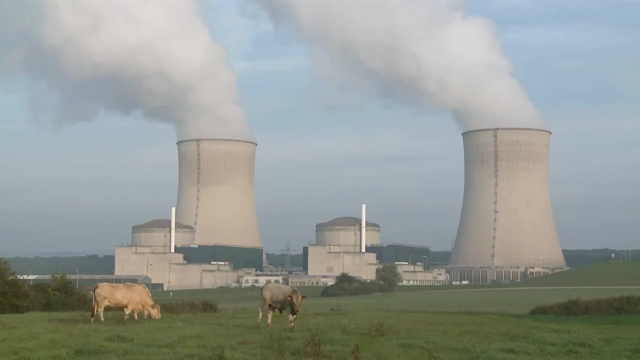 Over the past five decades, nuclear power has prevented the release of 50 gigatons of carbon dioxide. That's equivalent to two years of total global energy generation related emissions. Nuclear power is the most powerful tool at our disposal to stop human driven climate change in its tracks. Yet powerful industrial countries like Germany have turned 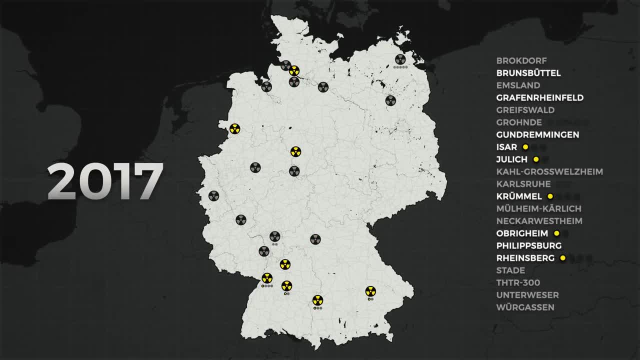 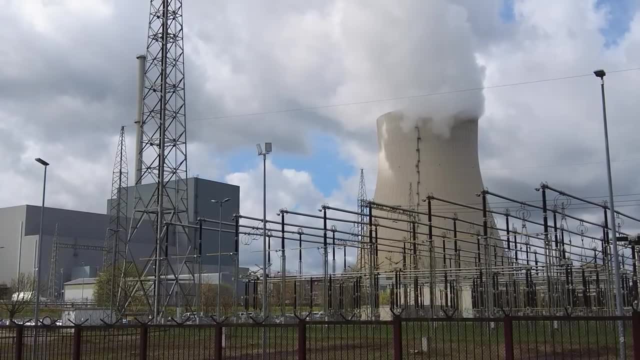 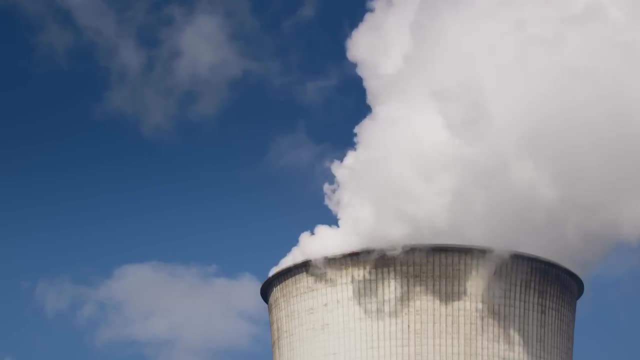 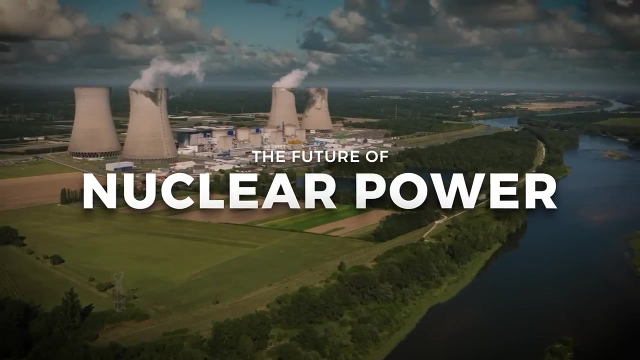 their back on this technology, rapidly deactivating power plants prematurely. Nuclear power, despite its clear climate change fighting potential, carries inherent risks that have hampered political will to invest in the technology. In order to thrive and help our planet overcome its greatest challenge, nuclear power needs to evolve. This is the future of nuclear power. 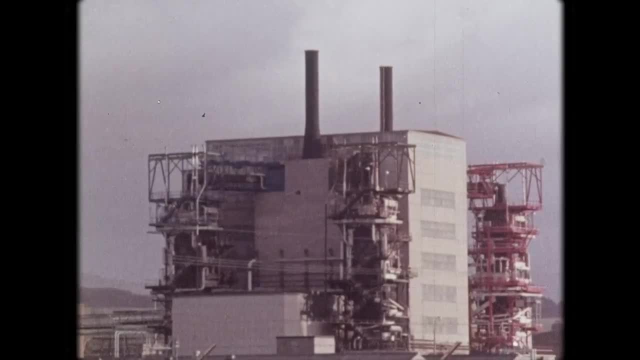 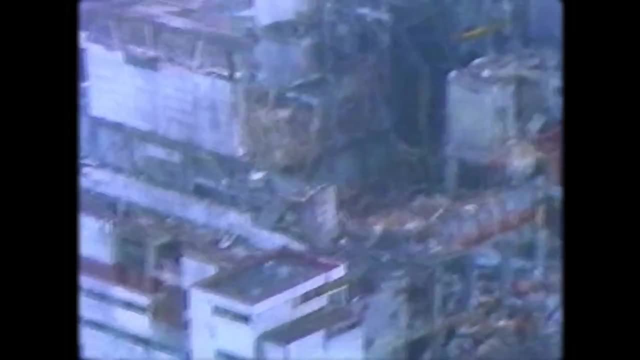 We can't begin to address the solutions of the future without addressing the failures of the past. Many of the most notorious nuclear meltdowns were caused by errors in coolant systems. Take the Three Mile Island partial meltdown incident of 1979.. The incident began. 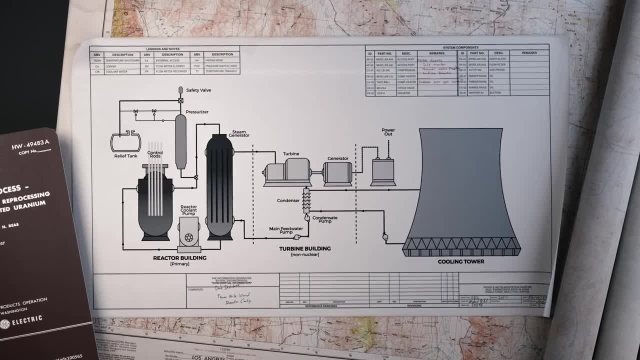 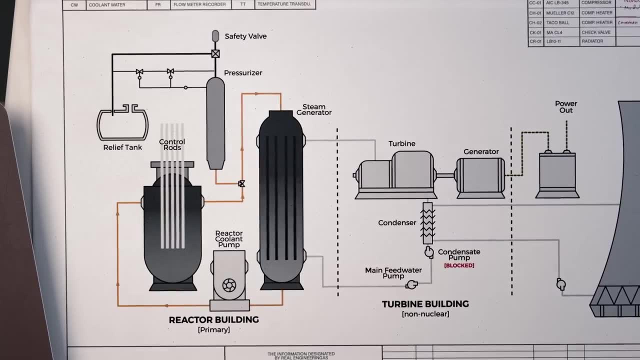 with a mechanical failure in the plant's cooling system. It all started when the steam generator stopped receiving water due to a faulty, clogged filter. The loss of water meant that the reactor's energy didn't have anywhere to go, raising the temperature of the reactor. 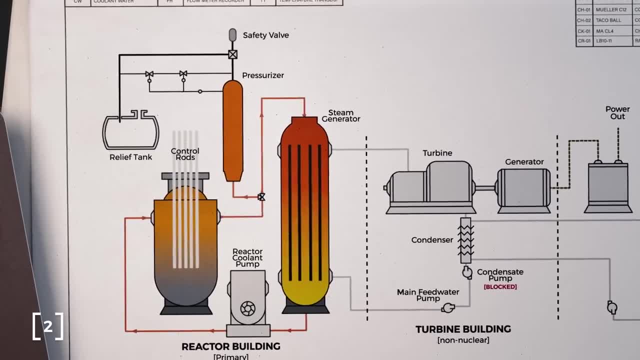 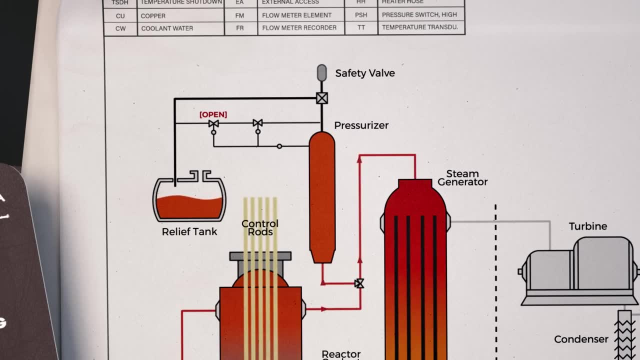 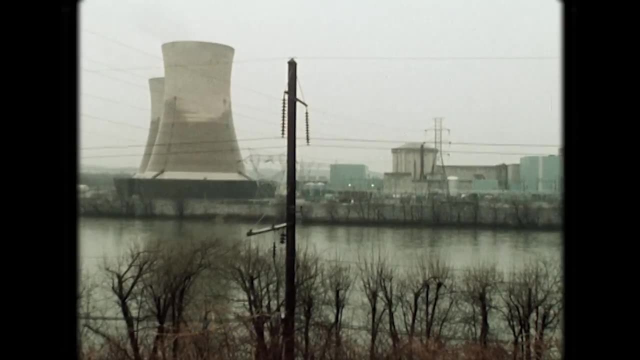 As the pressure rose due to the water being boiled, a relief valve opened, A valve designed to only open for 10 seconds. But another fault resulted in the valve staying open, allowing the precious coolant inside the reactor to escape, pushing temperatures even higher As the core temperature continued. 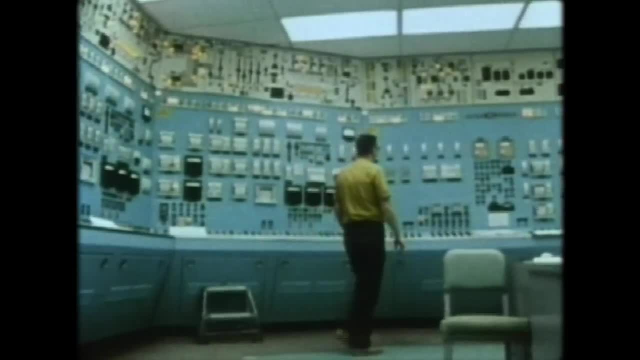 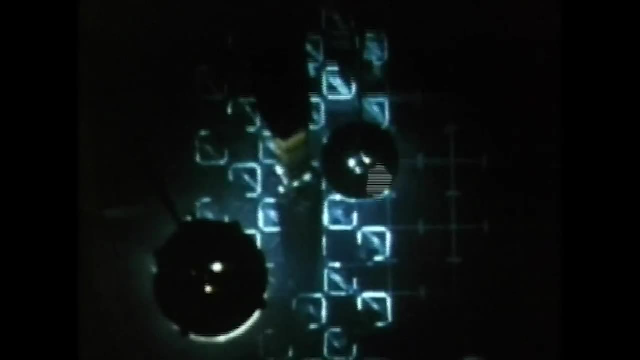 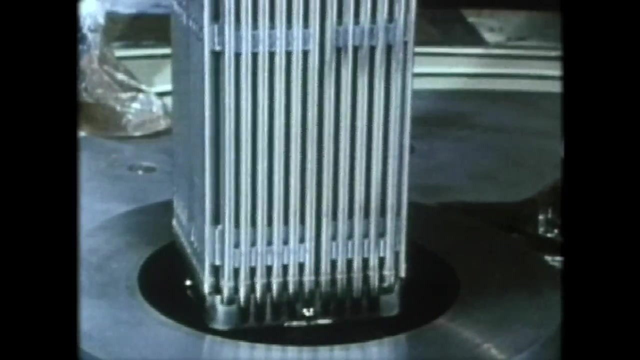 to rise. the reactor operators received conflicting information from the control room. The emergency water system that should provide extra water to the cores was blocked. Two days earlier, the plant was closed due to maintenance and the valves from the emergency coolant were closed. Unfortunately, they were closed. 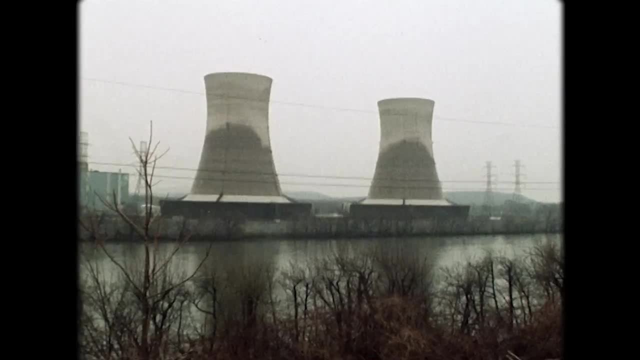 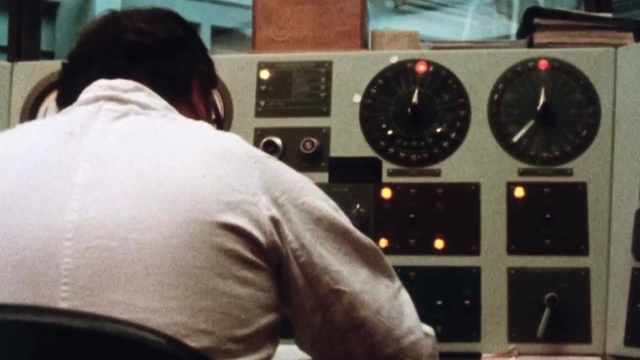 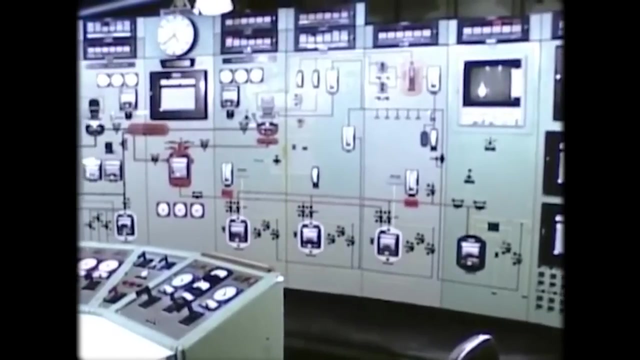 They were not reopened. when the reactor was restarted, The operator should have noticed that these valves were closed, but for unknown reasons he didn't see the warning lights on his control panel. One leading theory is that his stomach blocked his view of the control panel. Even then, the NRC, the regulatory body governing nuclear safety, had a rule that 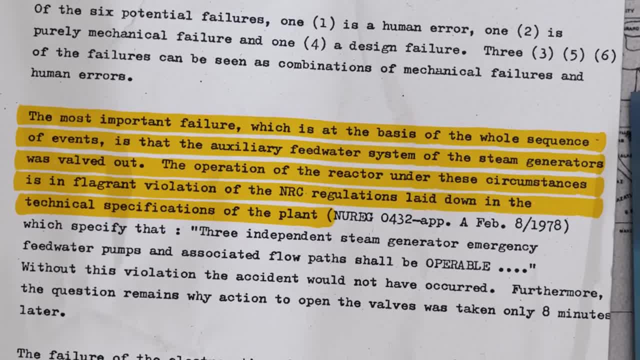 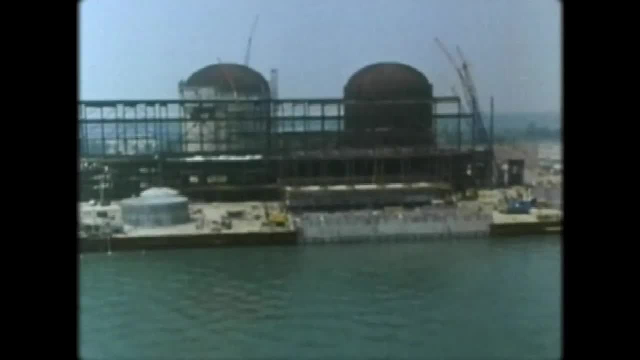 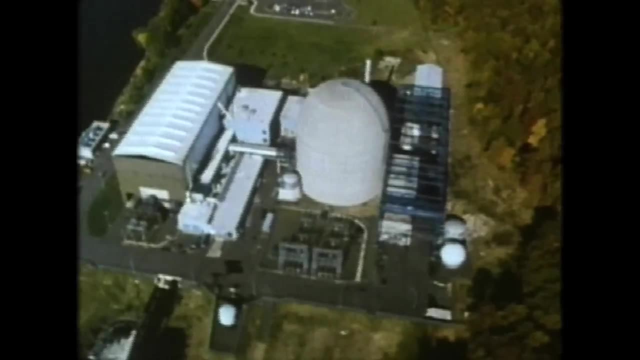 if the emergency coolant valves were closed, the reactor must be shut down. The situation at Three Mile Island was in clear violation of those rules. While the meltdown was triggered by a mechanical failure, the situation was worsened by human error. The Three Mile Island incident serves as a reminder of the critical importance of 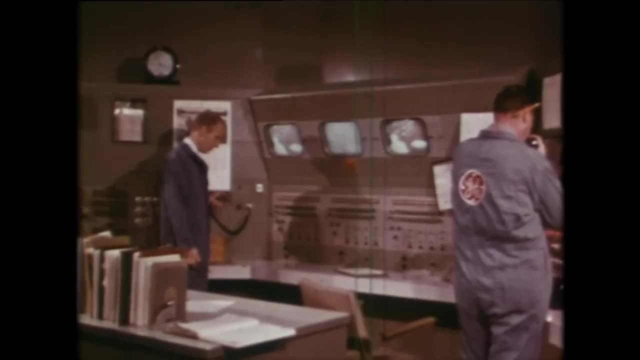 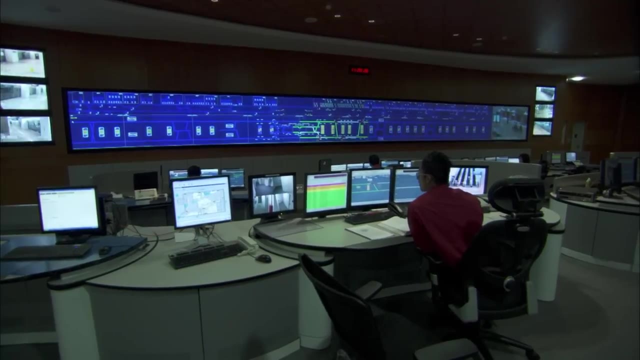 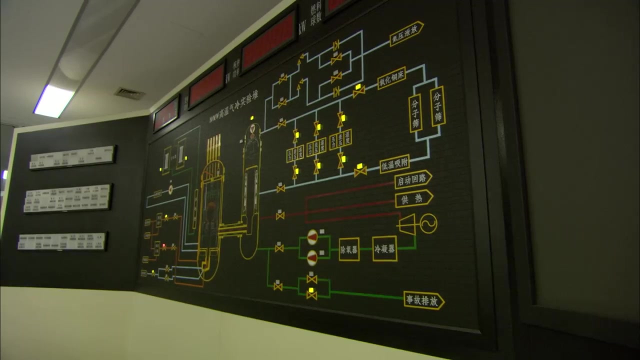 both robust mechanical safety systems and foolproof controls in nuclear power plants. It highlights the need for attention to detail in design, where even minor aspects like the positioning of alarms on control panels can have far reaching consequences, potentially fatal. To prevent such incidents, future nuclear power plant designs must proactively 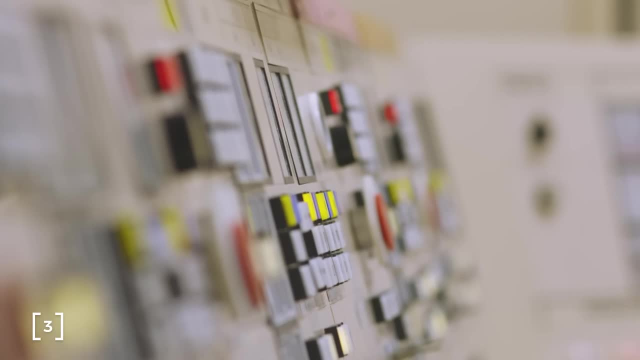 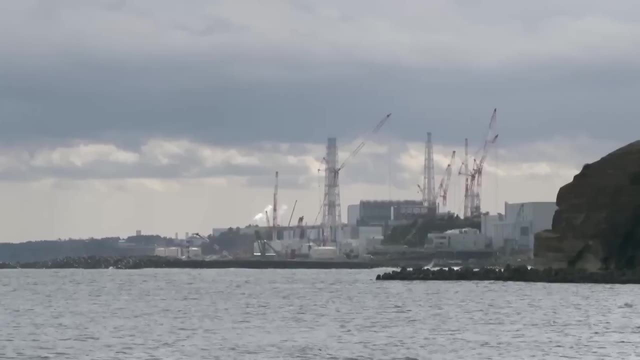 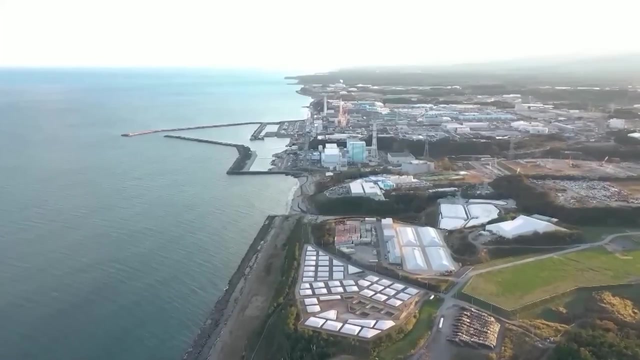 address these issues When the consequence of human error are nuclear meltdowns. there is no room for human error. In Fukushima, an earthquake and its resulting tsunami knocked out the plant's cooling systems. The cooling systems in Fukushima depended on a separate energy source, The 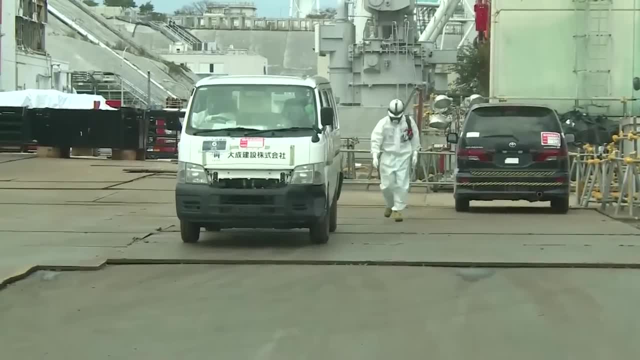 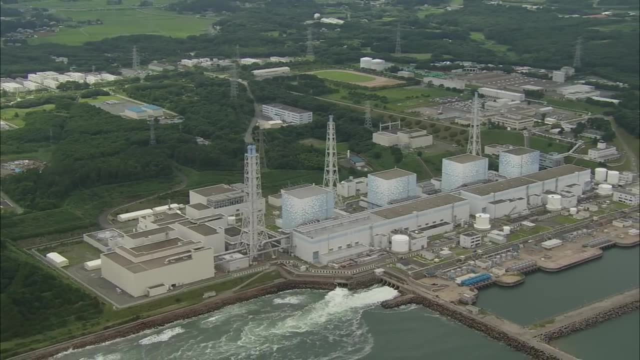 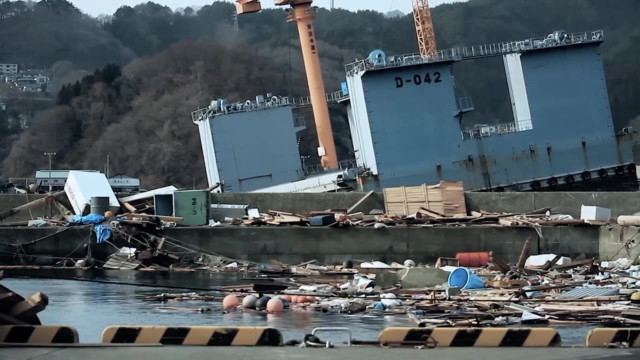 pumps that were needed to cool the reactors lost power, resulting in a catastrophic meltdown. The plant did have a backup system, which also failed. This need for external power to cool the reactors was a key disadvantage of this design. Fukushima also highlighted a weakness of current nuclear reactors: the use of water. 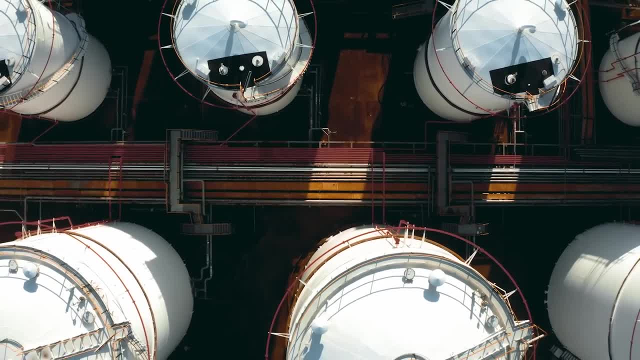 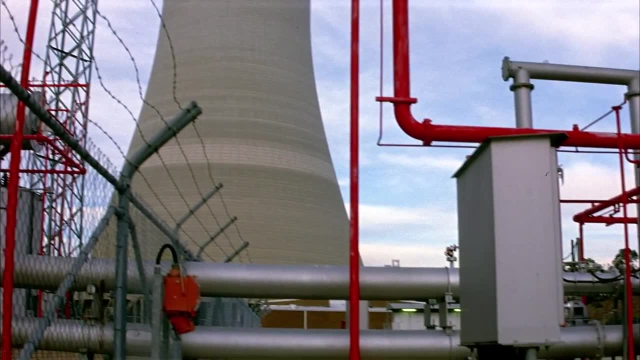 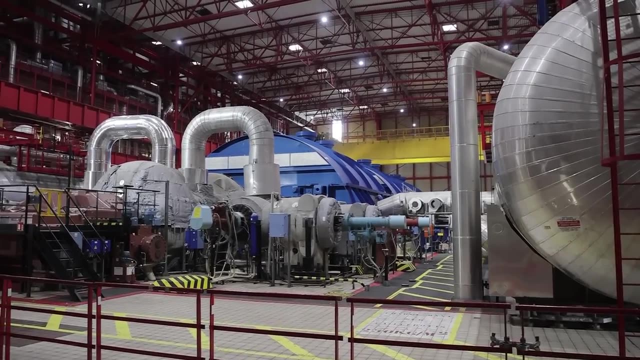 as a coolant. Liquid water is a great conductor of heat and serves as a fantastic cooling agent. However, when control is lost, this water can lead to high pressure steam explosions, spreading radioactive materials across vast distances. For this reason, many new reactor designs seek to incorporate passive cooling systems. 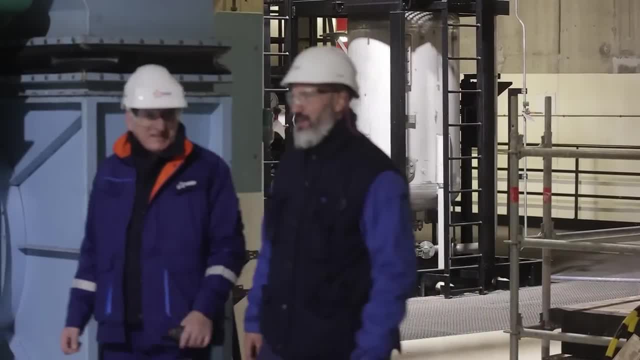 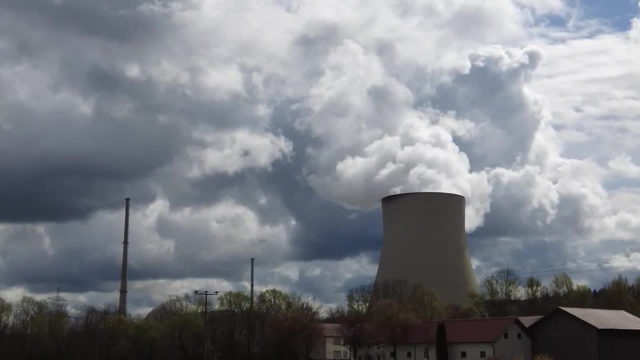 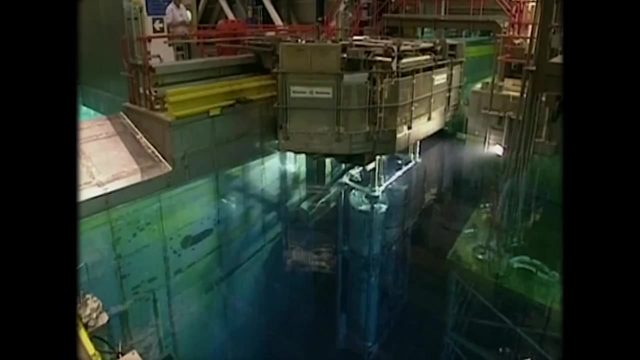 which require no external power source and aim to replace water with safer cooling mediums. Before discussing these future designs, there is another large problem facing nuclear energy: It's waste. Light water reactors operate in what is called an open fuel cycle In this. 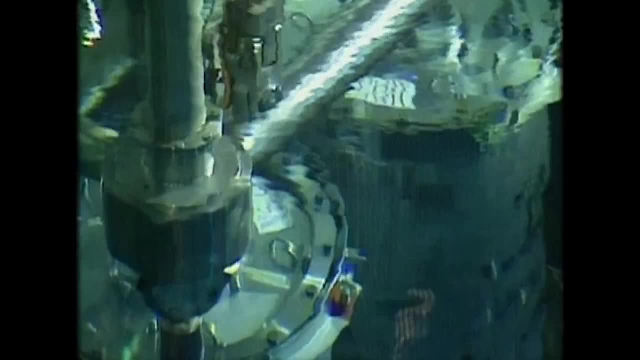 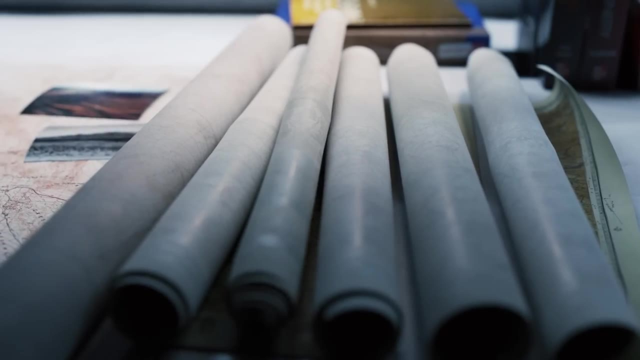 cycle, the uranium gets mined properly Processed, enriched, used and then stored, leaving us with barrels of radioactive waste that governments have been struggling to deal with. In the US, there have been plans to create deep geological storage facilities: 660 meters. 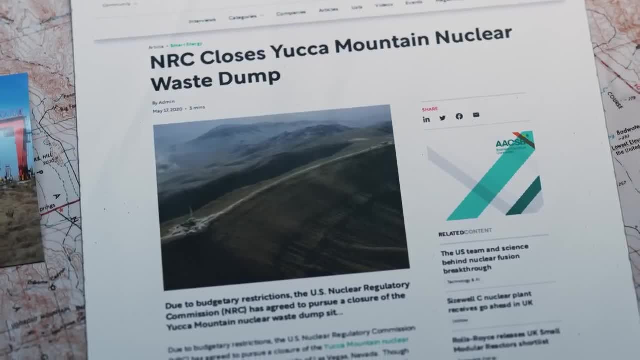 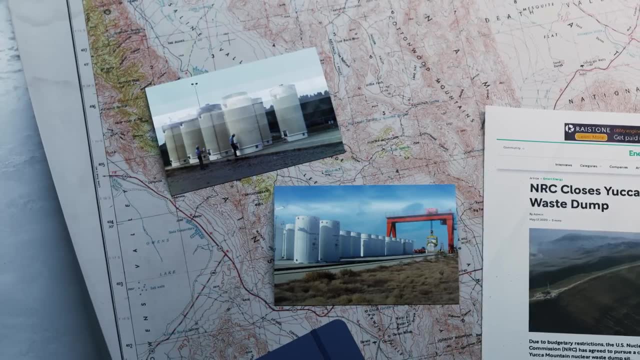 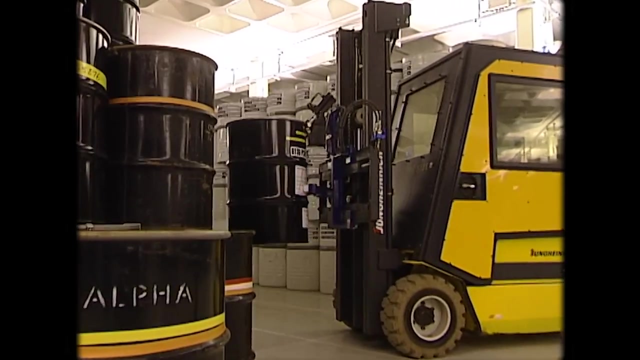 below Yucca Mountain. This has been the plan since the 1980s, but hasn't been put into action, So nuclear fuel is being stored in dangerous interim storage facilities scattered around the country. As is the case with most nuclear energy projects, it has faced delays and a lack of funding. 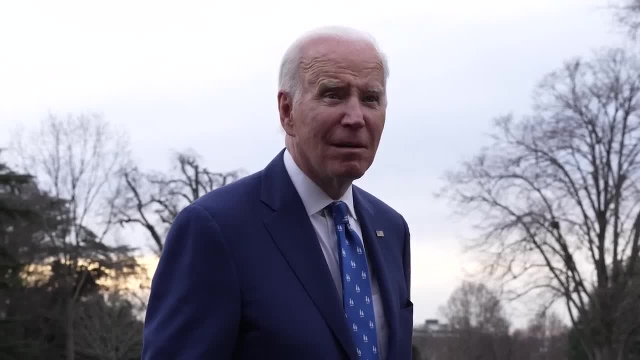 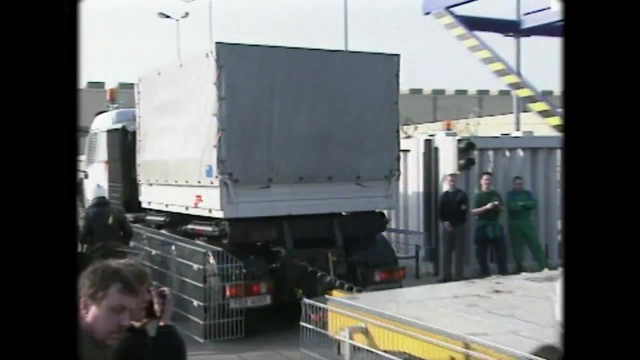 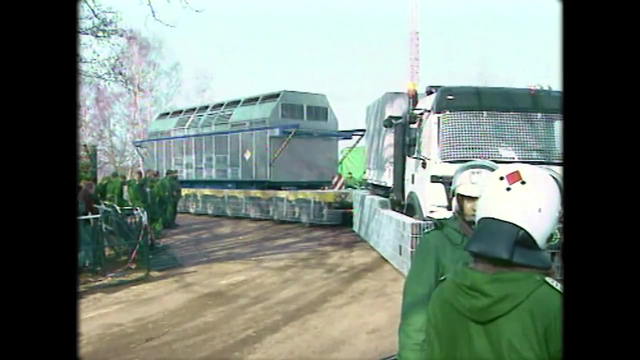 Obama, Trump and Biden have all failed to address this looming ecological threat. Waste management issues have continually caused political turmoil. Shipments of nuclear waste from France to Germany have been met with thousands of protesters, A key driver of political pushback on the development of nuclear energy. 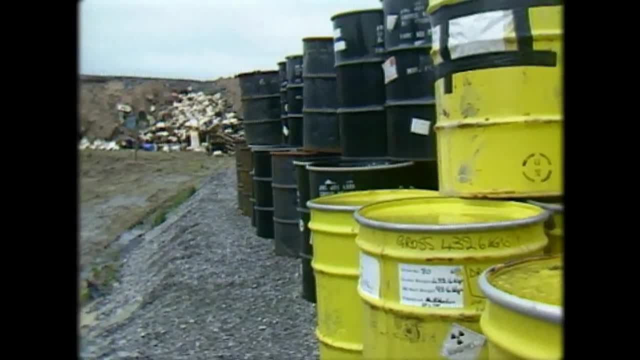 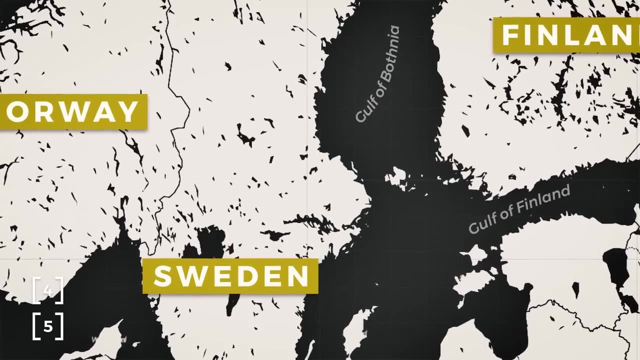 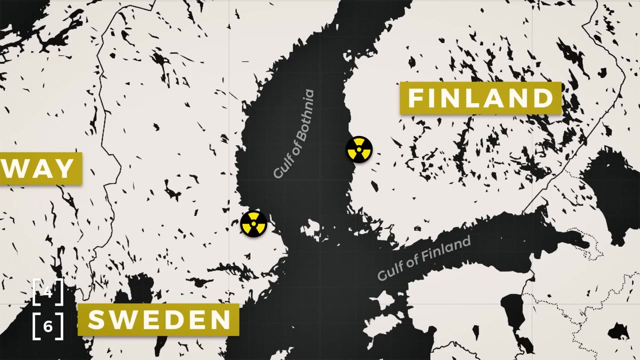 So is there an engineering solution to this logistical concern? Let's find out. Of course, adequate long-term storage is possible. Sweden has approved large storage repositories here in Frostmach. Finland has made similar arrangements to store its nuclear waste here. This Finnish deep geological repository is expected to come online within a year. 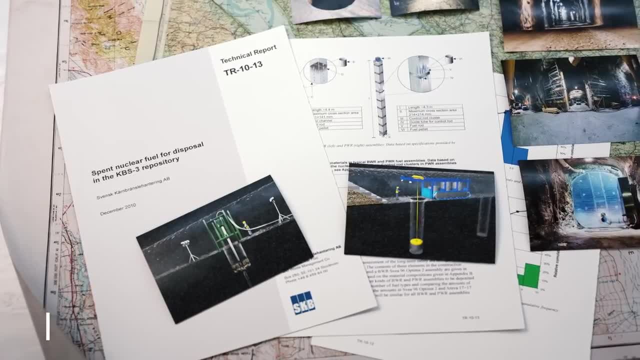 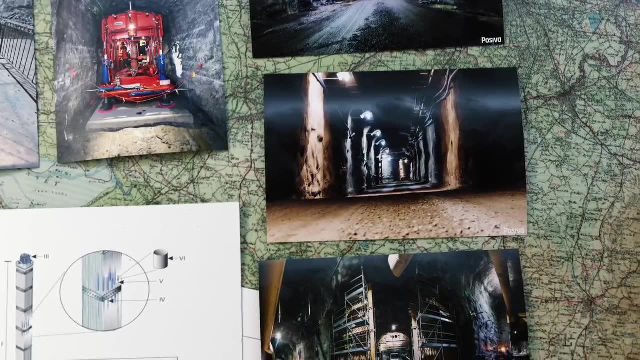 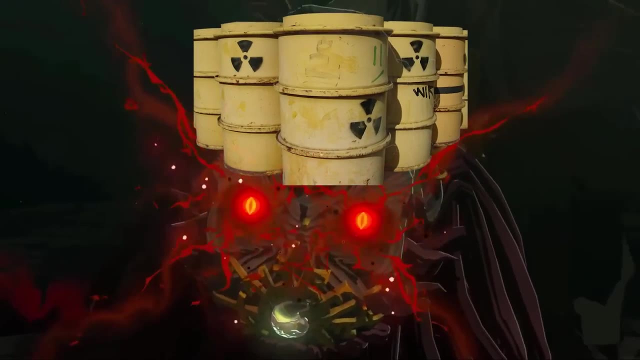 Deep geological repositories are sophisticated engineered systems that employ multiple layers of protective barriers to isolate the spent fuel from the surrounding environment. What if we could make use of this, Rather than locking it away for centuries like some sort of supernatural Zelda villain? nuclear waste can be recycled. 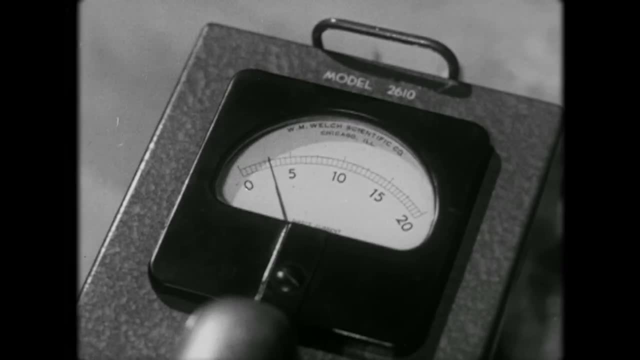 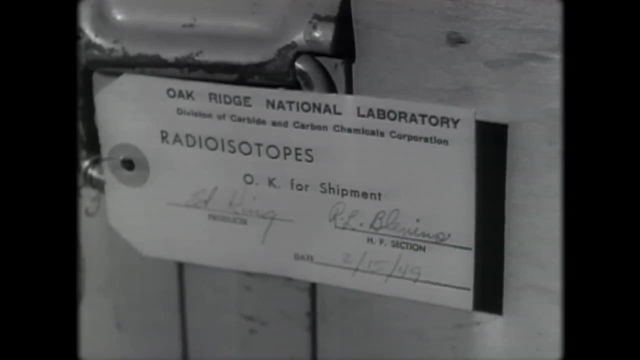 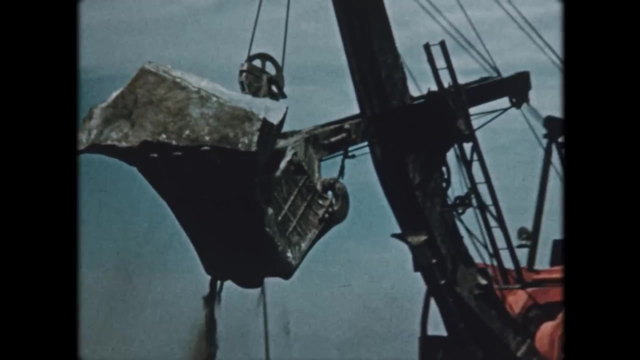 During the early development of nuclear power, uranium was thought to be a limited resource, So a lot of research was directed into creating closed fuel cycles where the spent uranium would be reprocessed and recycled. But the assumption of limited uranium was wrong. Uranium is very common in the Earth's 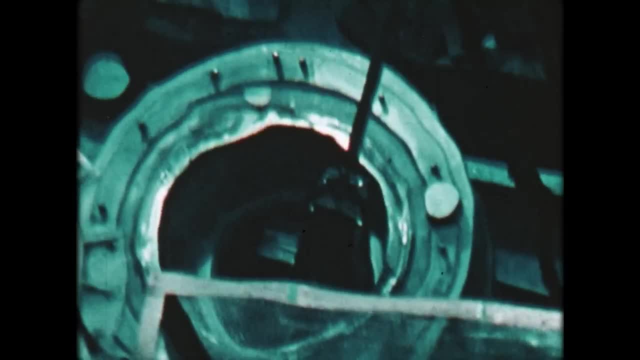 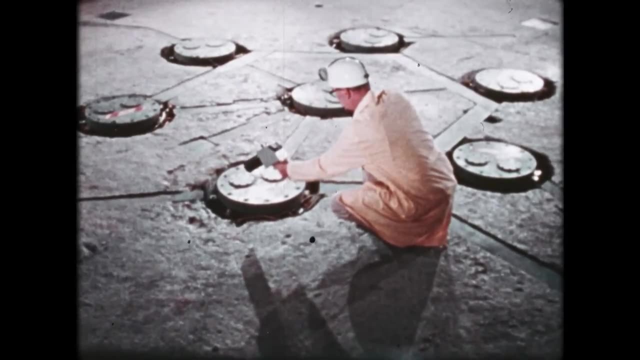 crust. It's much cheaper to produce it before it's too expensive. That means it's less cheaper to mine, enrich and process uranium than it is to recycle nuclear waste into workable fuel. Hence the adoption of the open fuel cycle. This is the system currently operating on most nuclear reactors with new waste piling. 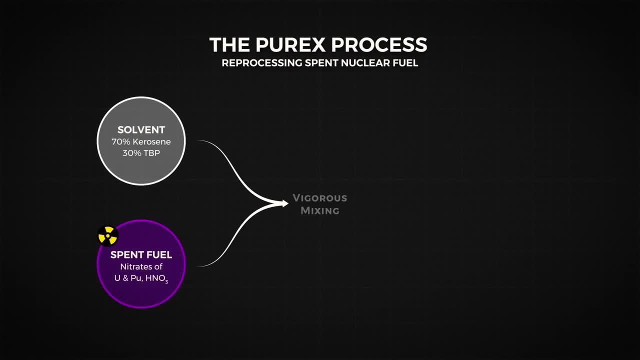 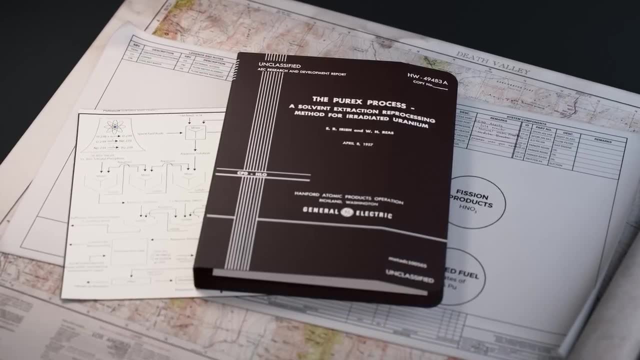 up every minute. Recycling spent nuclear fuel is just a matter of separating unused uranium from the fission products. This process is not new. it was developed in the 1950s and the basic steps are still used today in France and Japan. 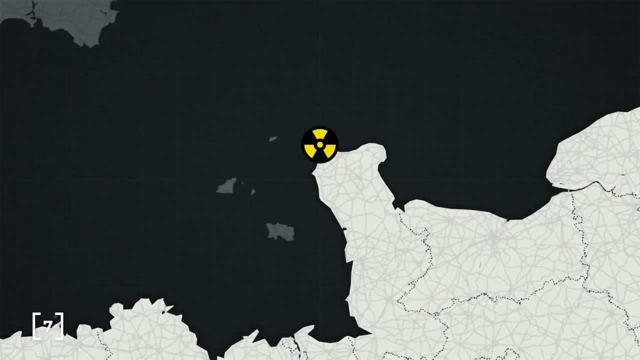 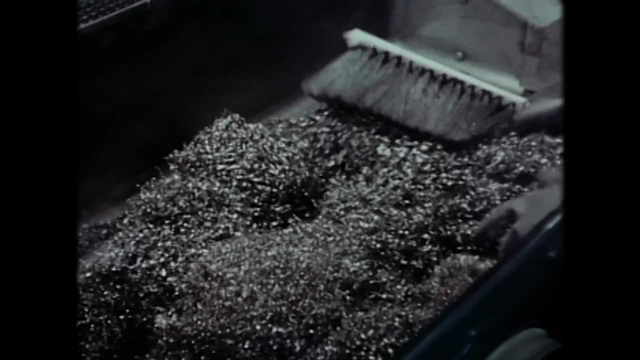 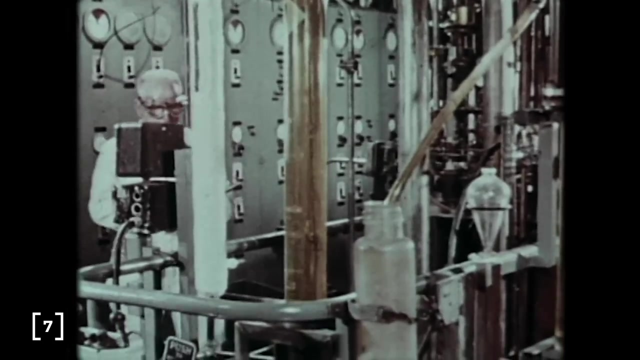 France, for example, cools its nuclear waste here. for three years it sits there before moving to the reprocessing steps, With the added cost and the potential of extracting plutonium for nuclear weapons. the Carter administration banned US recycling facilities in 1977. 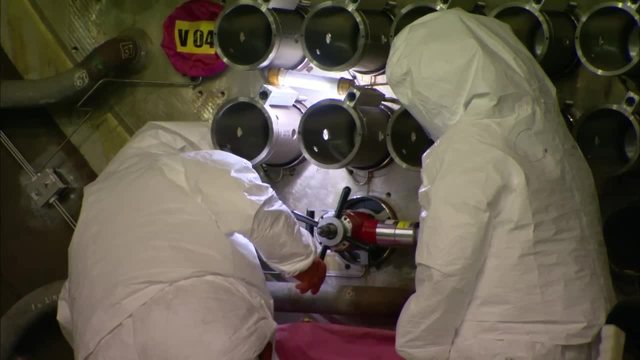 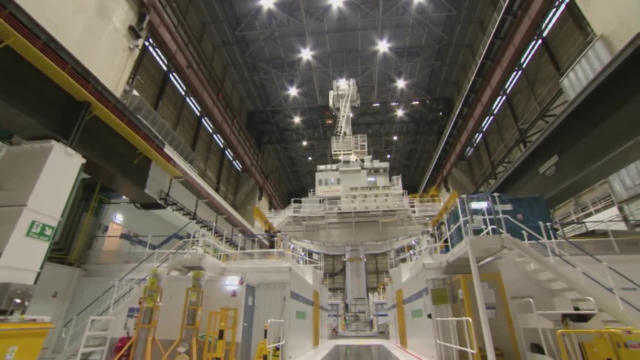 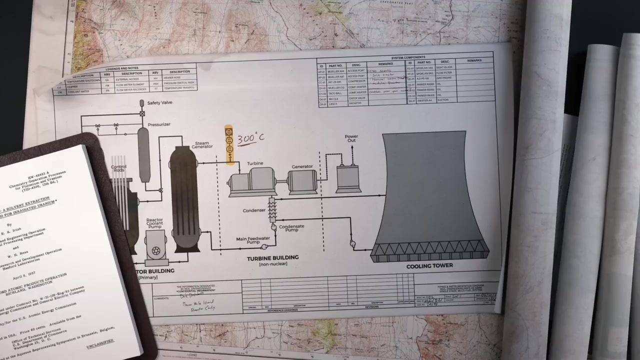 This recycled fuel can go back into regular light water reactors or it could go into newer reactor designs. Two common themes in nuclear waste New generation reactors is passive cooling and high thermal efficiencies through high temperature coolants. Light water reactors are limited to operating at around 300 degrees celsius. 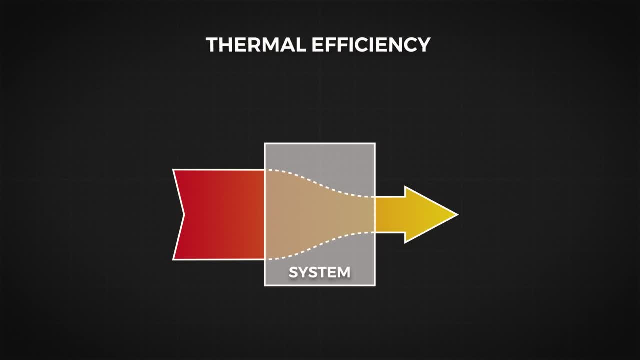 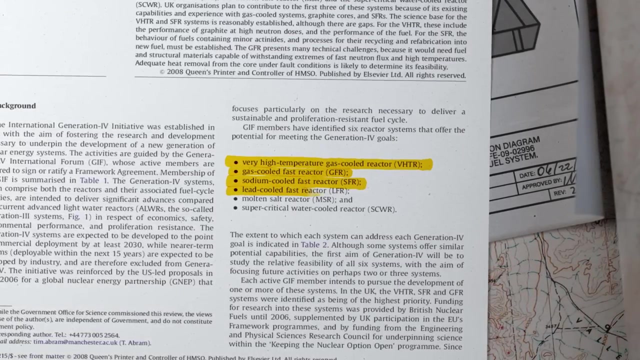 Above this temperature the high pressure water begins to boil. Thermal efficiency is how much electrical energy we can produce from thermal energy And in general this efficiency gets better with higher temperatures. To increase efficiency, future nuclear reactors can switch the coolant to something that can. 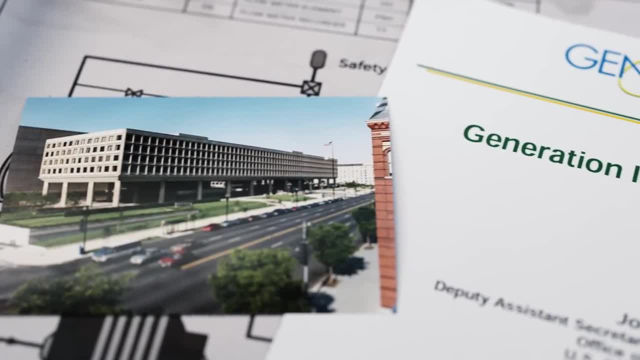 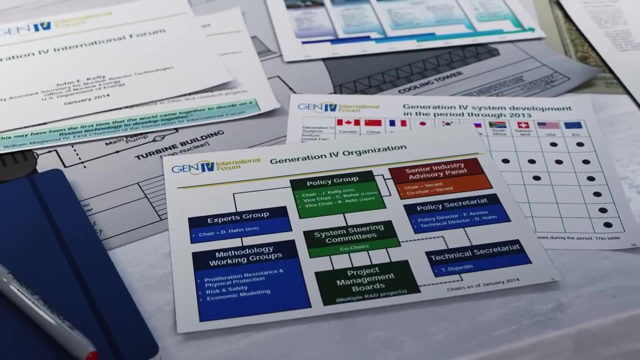 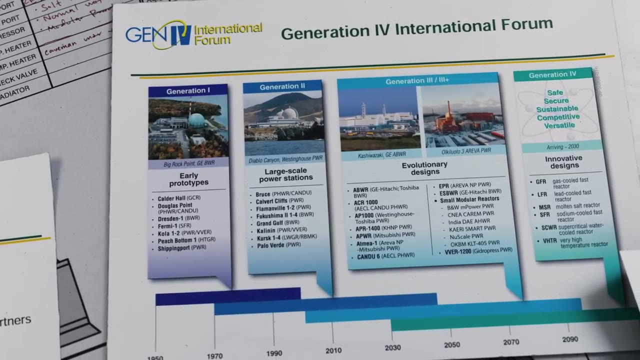 handle higher temperatures. In the early 2000s, the US Department of Energy decided to create the Gen 4 International Forum. It was composed of the best scientists from around the world to direct policy decisions and funding for new reactor designs. They chose a total of six new reactor technologies and coined them Generation 4 Reactors. 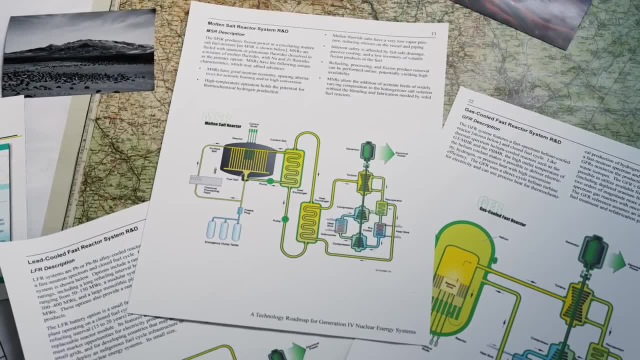 Instead of using water as a coolant, Gen 4 reactors can use gas, supercritical water, molten salts, molten lead or solar energy. They can also be used as a nuclear reactor. In the early 2000s, the US Department of Energy decided to use sodium to increase the operating. 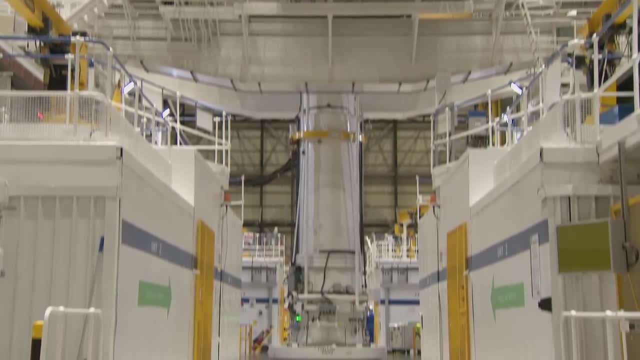 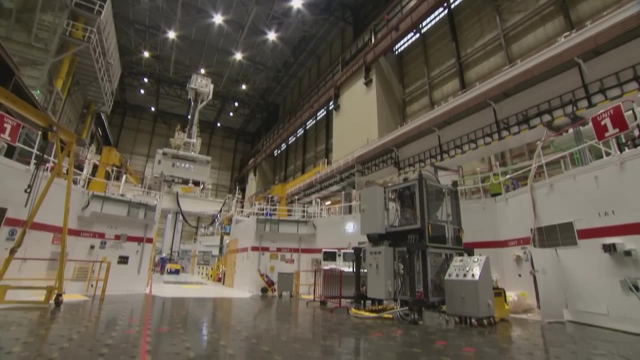 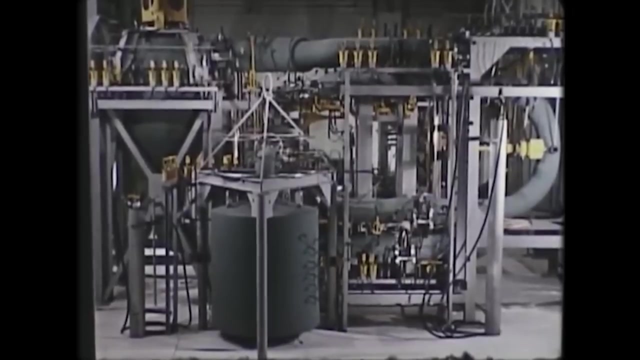 temperature of the reactor. This increase in efficiency will result in less nuclear wastes per gigawatt generated, But these designs also aim to increase passive cooling capabilities and limit nuclear proliferation risks. One of the most interesting prospects is the Molten Salt Reactor, or MSR. 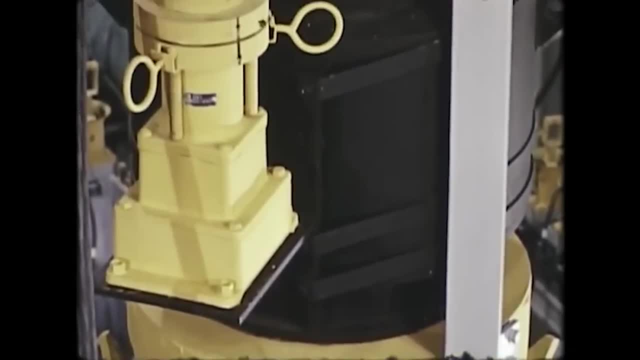 In these reactors, the coolant and the radioactive fissile material are all combined. The basic premise of these reactors was tested and the results are as follows. The first reactor to be tested is the Molten Salt Reactor, or MSR. In these reactors, the coolant and the radioactive fissile material are all combined. 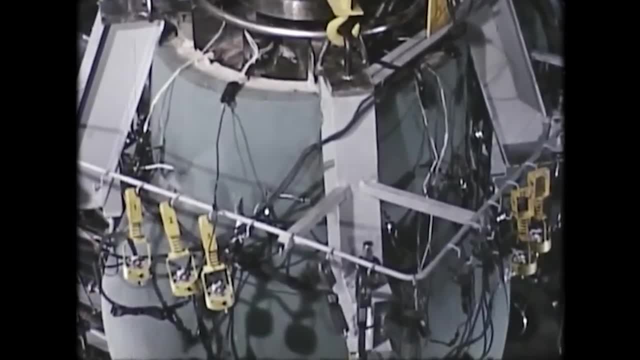 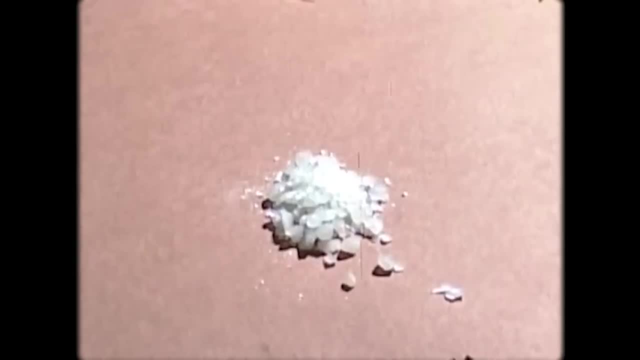 Here is what is being tested and experimented with during the 1960s at the Oak Ridge National Laboratory In a molten salt reactor. the fuel consists of nuclear fuel such as uranium or thorium dissolved in a molten salt mixture. 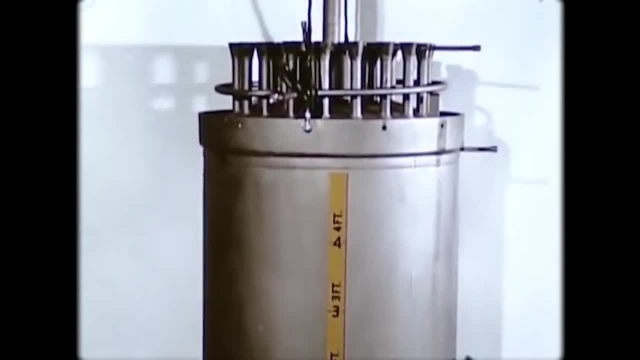 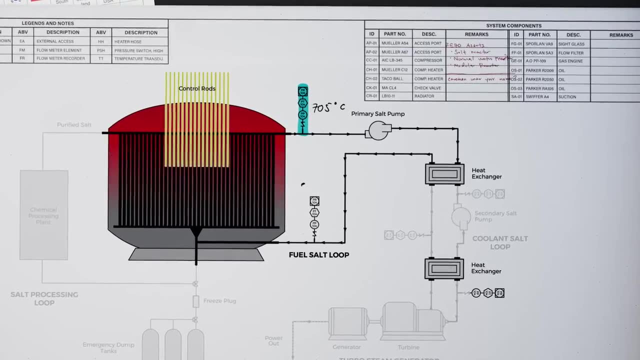 The salts typically use their fluorides or chlorides, which have high melting points and good heat transfer properties. The fuel salt circulates through the reactor core, absorbing the heat generated by the nuclear fission. After it passes through the core, the fuel salt goes into the reactor. 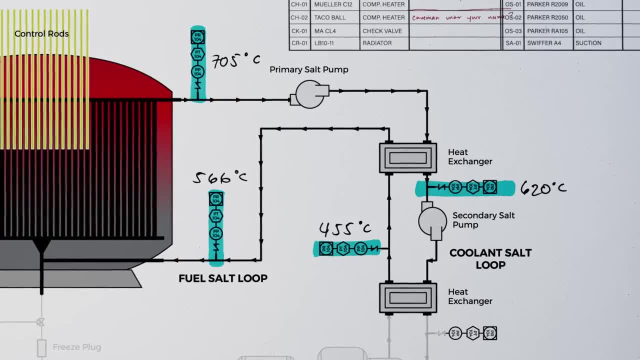 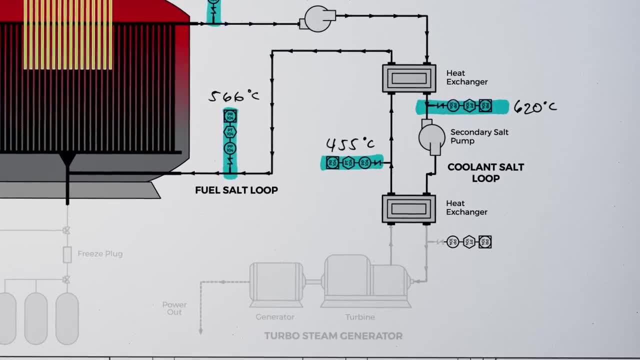 At this stage the 不要 deteriorates and would damage the reactor's principles. transfers heat to a secondary salt coolant loop. The secondary loop, which does not contain fissile material, absorbs the heat from the fuel salt and carries it to the heat exchanger. 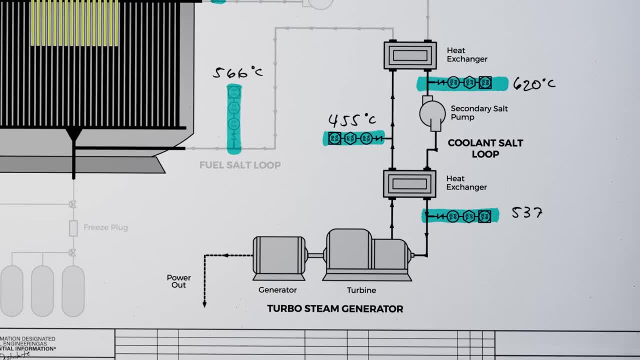 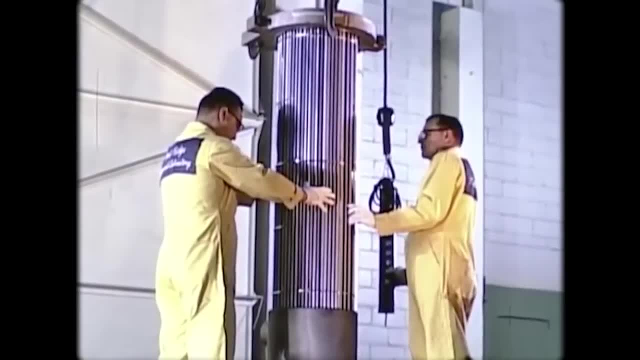 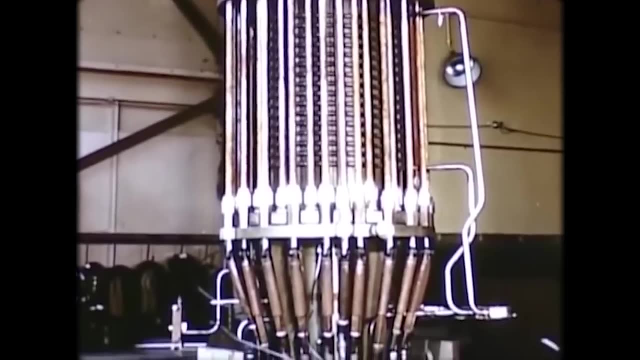 In the heat exchanger, the heat from the secondary salt is transferred to a separate working fluid, typically water, which then powers a steam generator, Since the coolant they use does not need to be at high pressure. like the water cooled reactors in Fukushima, salt reactors are not at risk of high temperature steam explosions. 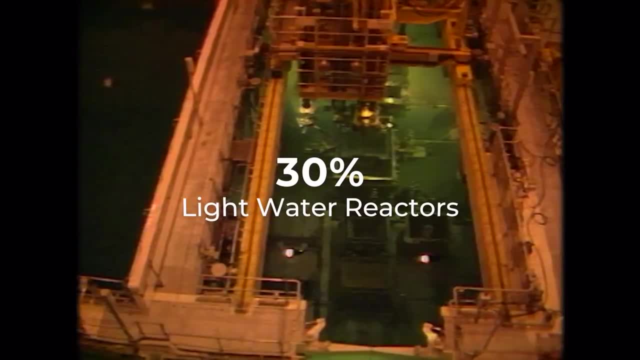 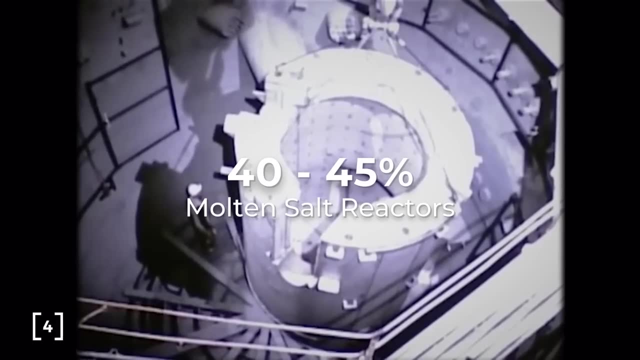 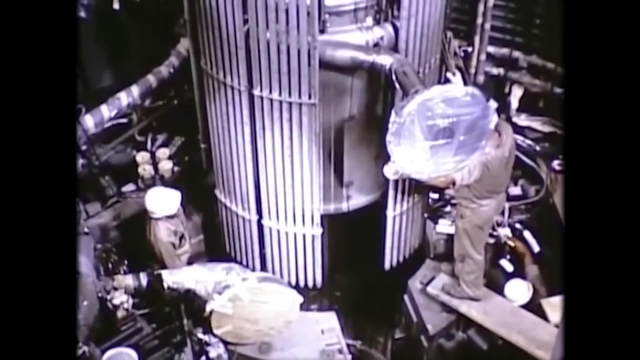 While light water reactors typically have a thermal efficiency of around 30%, Molten salt reactors have been theorized to achieve efficiencies between 40-45%. Molten salt reactors also have the potential for inline fuel processing, which means that while the reactor is operating, the fuel salt can be continuously reprocessed to remove. 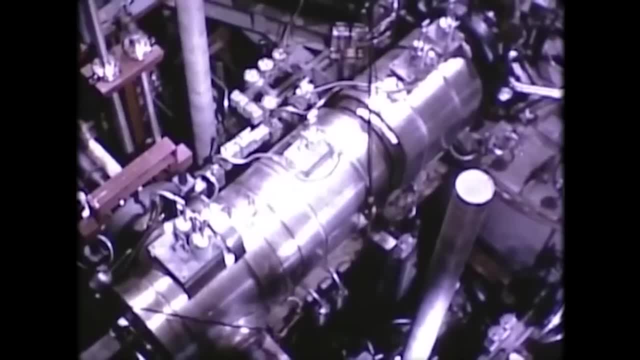 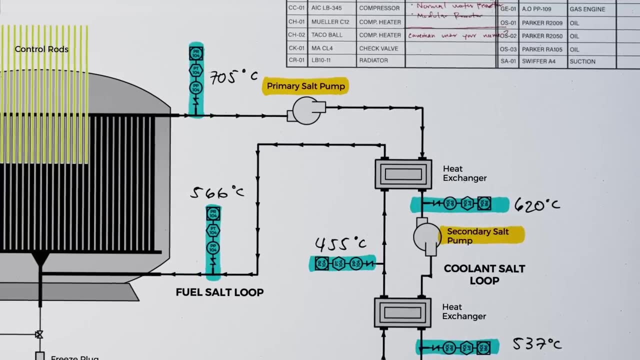 fission products and add new fuel Meaning, the machine can run continuously- continuously without stopping for refuelling. At first glance, you'll notice that the system needs not one but two pumps. However, these reactors can safely cool down even when power is lost to these pumps. The salts chemical properties naturally inhibit further nuclear fission as temperatures increase. The exact mechanisms of this depend on the salts composition, but generally as the molten salt gets hotter it expands. This expansion decreases the volume of fuel in the core of the reactors and therefore decreases the rate of nuclear fission, Meaning the hotter. 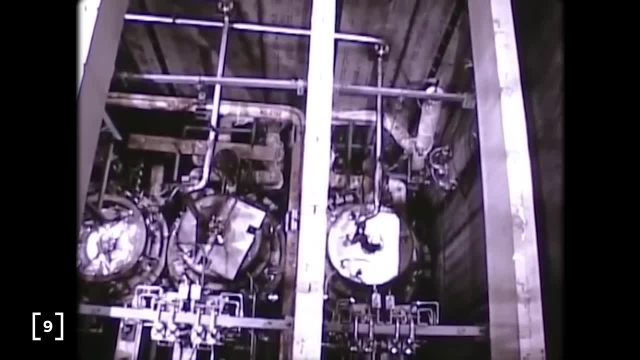 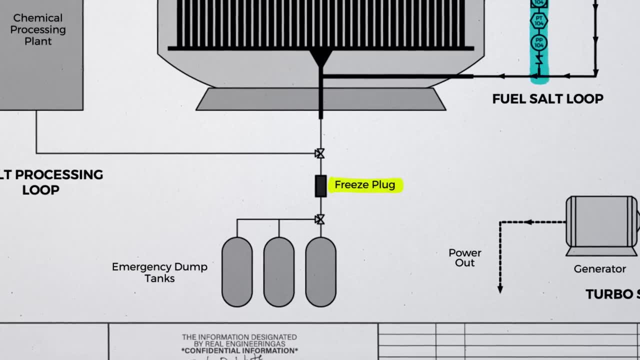 it gets, the less fission occurs, helping prevent nuclear meltdown. A freeze plug is also located at the bottom of the liquid salt pool. The freeze plug is designed to melt at a particular temperature In the event of an uncontrolled rise in temperature. 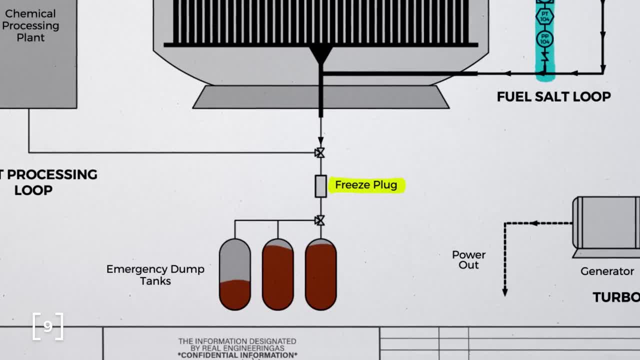 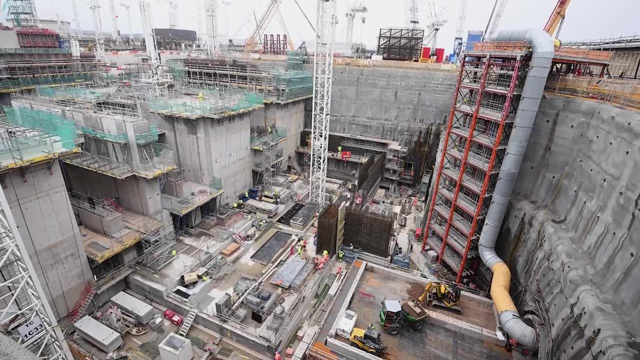 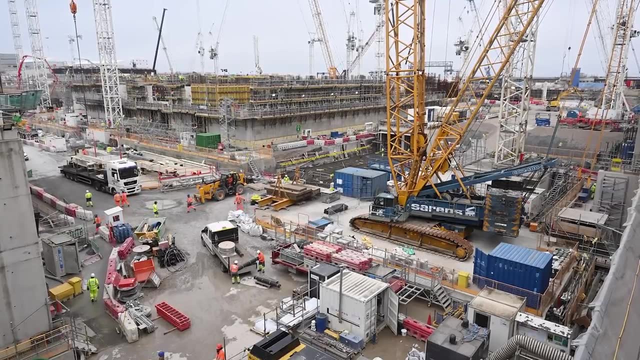 the plug will melt and allow the fuel and molten salt to pass through To passively drain into cooled dump tanks. Molten salt reactors are some time away from commercial readiness and that problem extends to all other 4th generation reactors despite significant support from proponents of these. 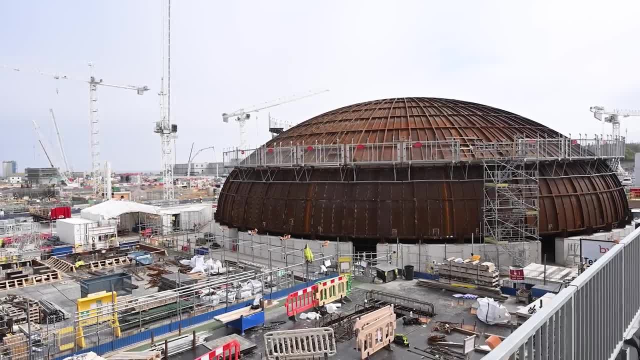 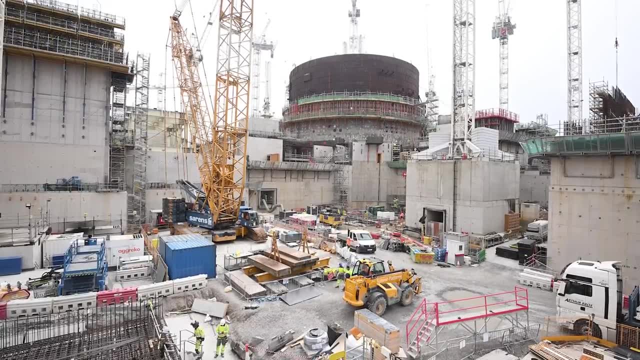 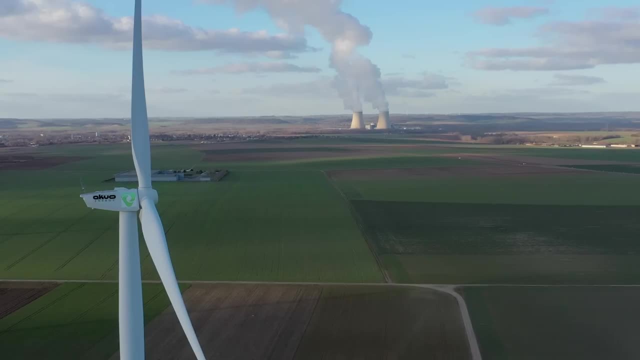 technologies. The 4th generation international forum originally proposed that most of these technologies would be ready by 2020.. But, based on the fact that the only footage available is from the 1960s, that has not come to fruition. Lack of funding and competition from low cost, solar and wind has held back development of 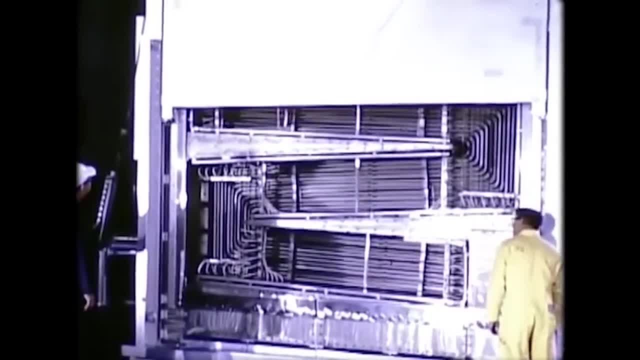 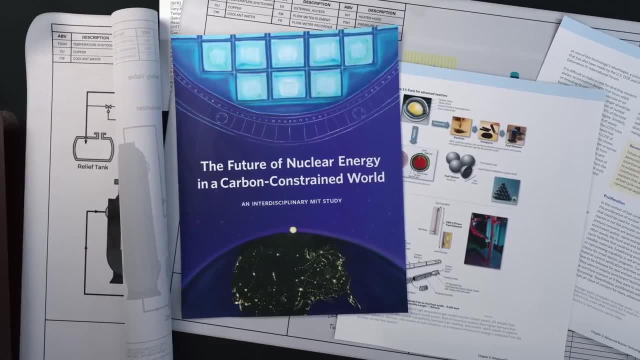 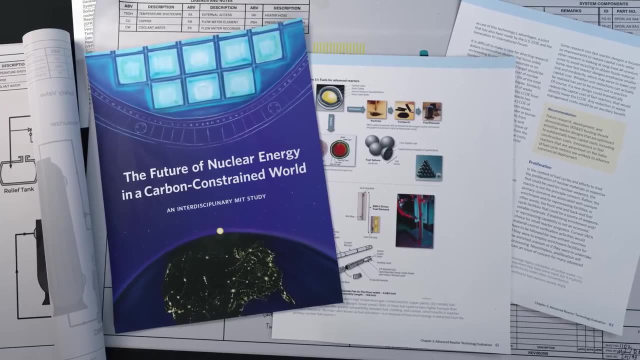 these 4th generation technologies. This problem is only going to continue until nuclear energy addresses its largest problem: cost. Since 2003,, MIT has been conducting studies specifically aimed at guiding researchers and policy makers towards a viable future for nuclear energy. In their latest report, 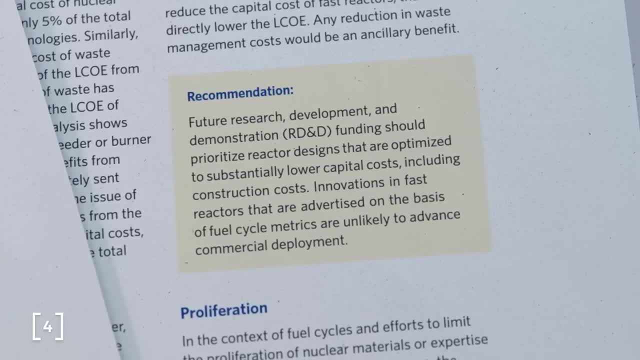 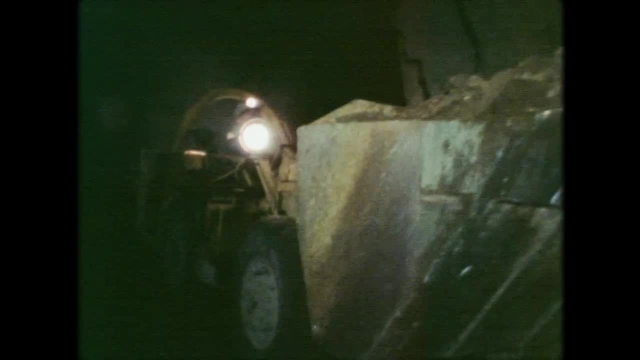 they stated that the utmost importance must be given to the use of nuclear energy in the given to lowering the cost of nuclear plants, And thus the most promising ideas seek to address these cost issues. While deep geological repositories, uranium reprocessing and gen 4 reactors had the brunt, 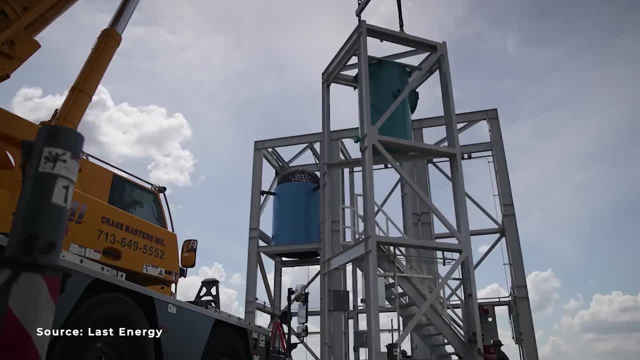 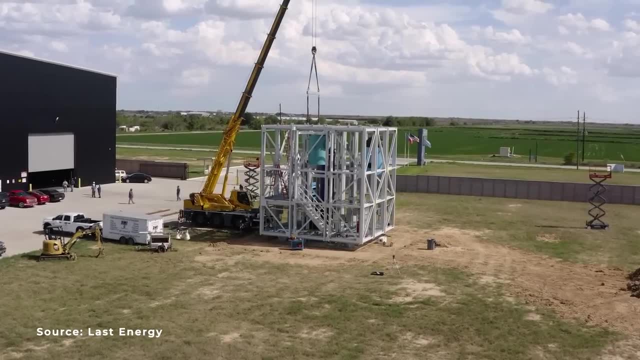 of work done during the 1900s, a new design concept started to emerge in the early 2000s: Small Modular Reactors, or SMRs for short. The goal of this design is to miniaturise reactors and convert them into small, standardised 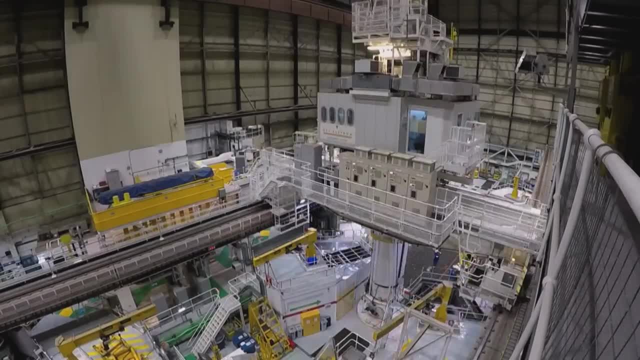 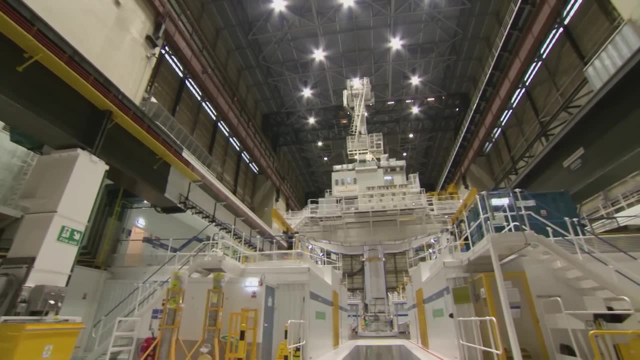 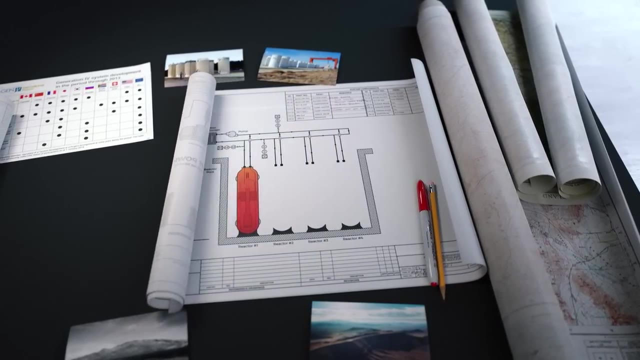 modules that can be fabricated in factories. This standardisation could not only decrease costs, but inherently increases their reliability and safety, as complexity is removed from the manufacturing and assembly, while decreasing on-site construction costs. Small modular reactors work in much the same way as regular nuclear plants, but with smaller. 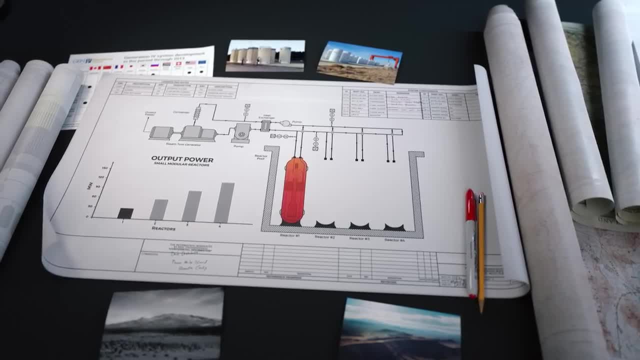 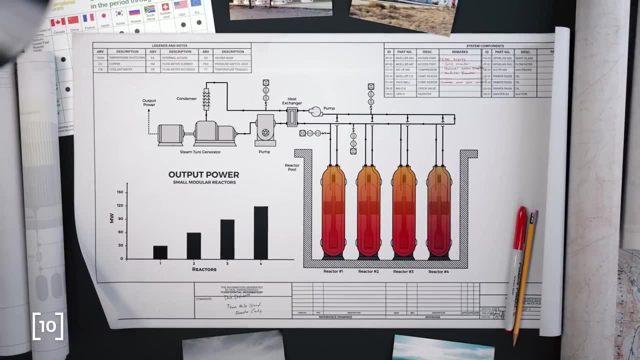 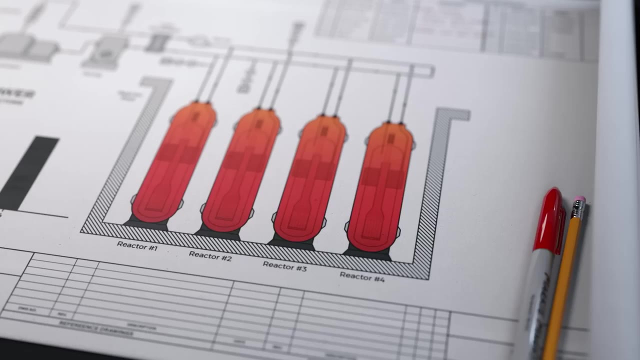 individual reactors that can work in expandable modules, Gradually increasing the output of a power plant with cheaper factory made modules, rather than building one large custom designed nuclear power plant with 1000 megawatts of electricity capacity. Making the reactor smaller also comes with the big benefit of passive safety. 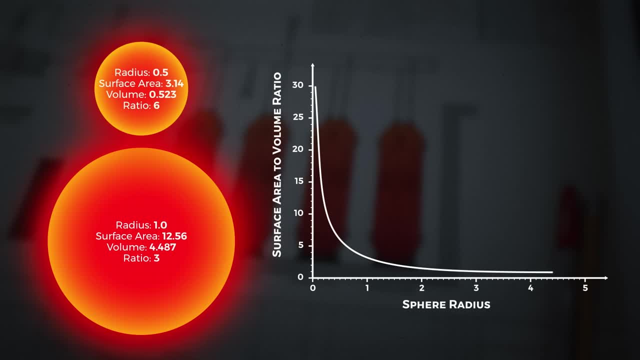 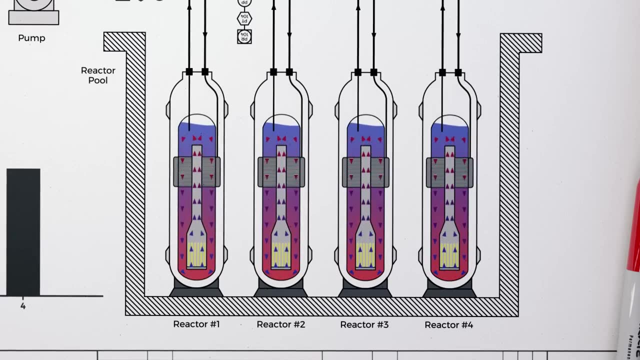 A smaller reactor has more surface area for heat transfer to occur in proportion to the volume of material that needs cooling, meaning natural convection cycles are sufficient to cool the reactor. As the coolant is heated, it rises due to its lower density, establishing a natural 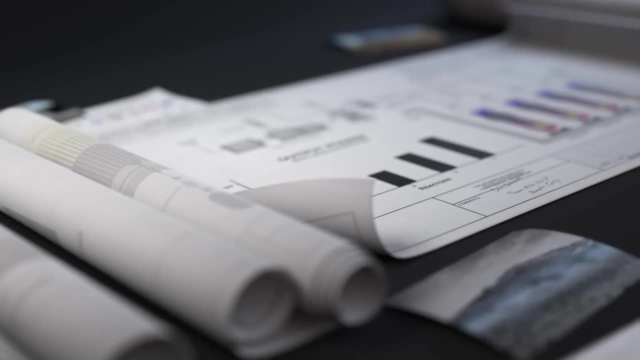 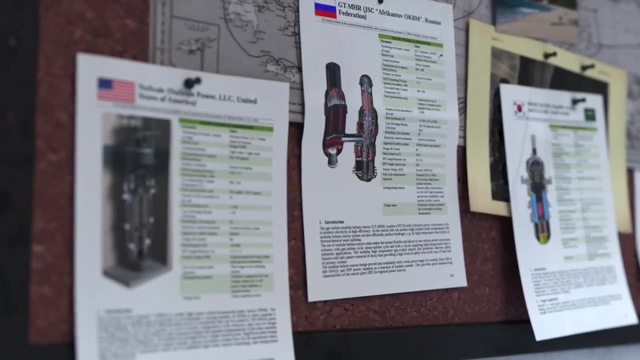 flow pattern. This drives the cooling process. SMRs are not defined as one type of nuclear reactor or design. rather, they are a family of designs that take advantage of the miniaturisation of the technology. Because of this, no one SMR is like the other. 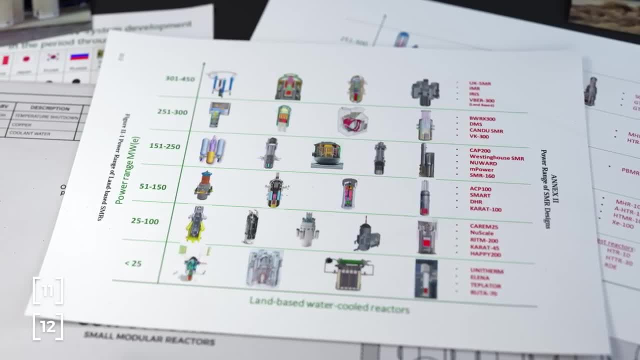 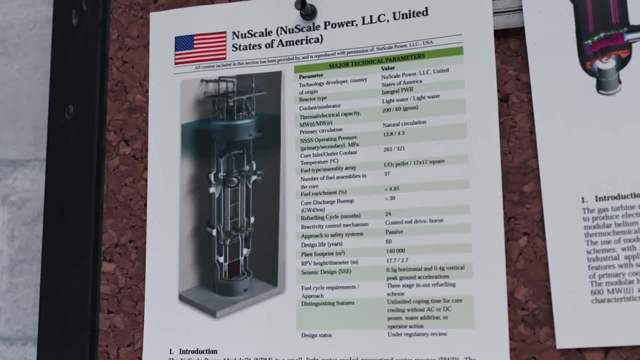 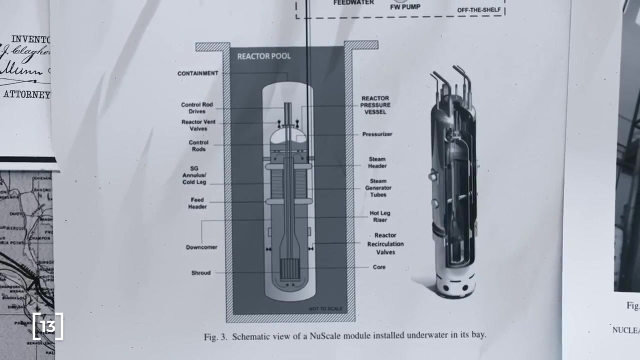 Some use Gen 4 reactors, others use light water reactors. Currently, over 70 commercial small modular reactors are being developed. NuScale may be the most promising of all these companies- Their most recent 70s and 90s. The 177 megawatt module is around 20 metres tall and 4.5 metres in diameter. 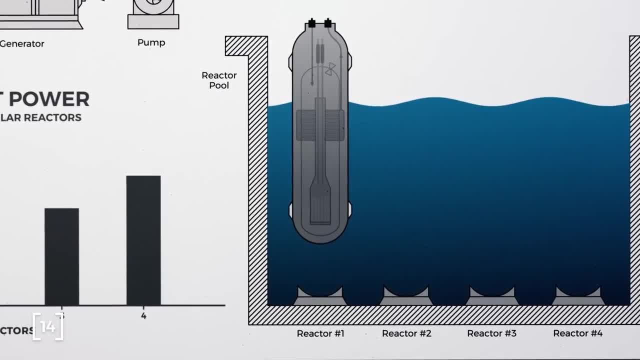 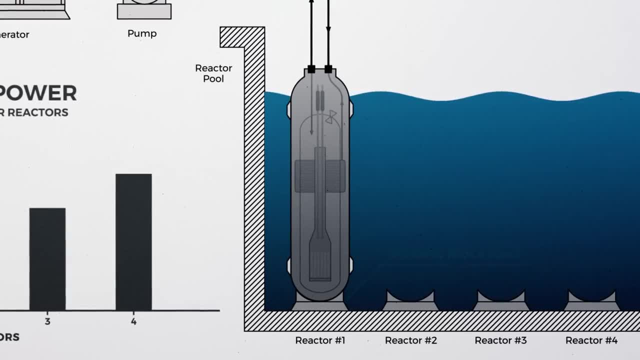 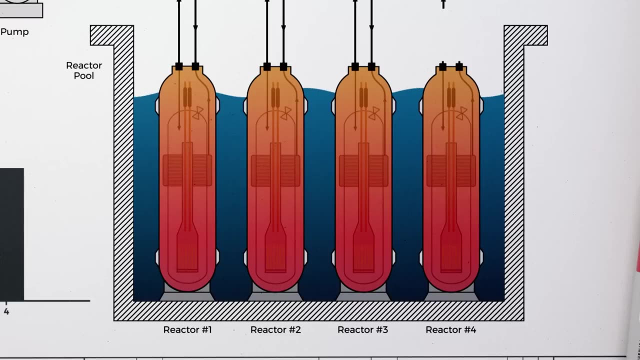 Each of these modules is lowered into a water bath and set on seismic isolators. This makes sure that any earthquakes do not affect the reactor. All of the components needed for the nuclear reaction are fitted in one steel containment vessel. To create a larger plant, multiple modules are connected together. 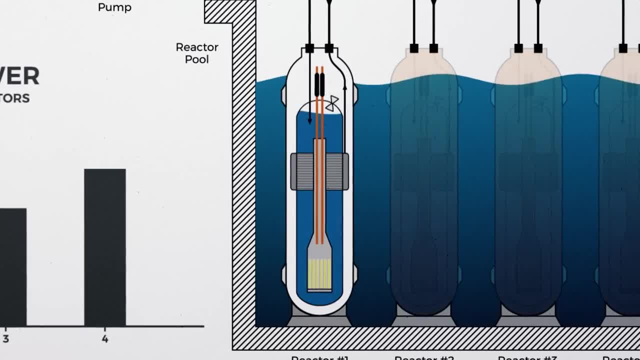 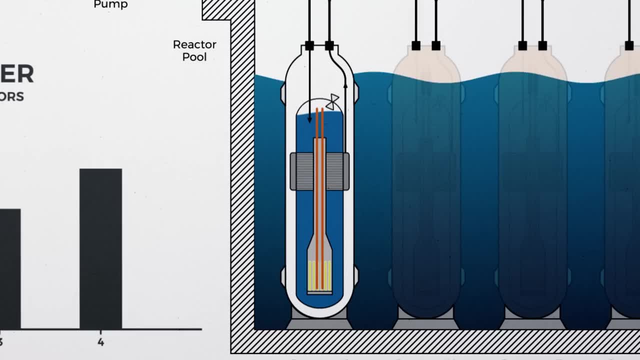 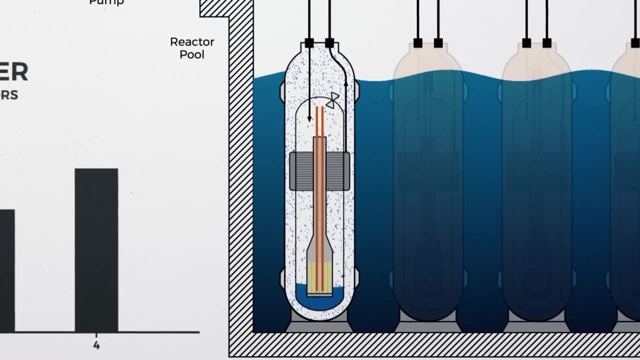 If power to the reactor is lost, control rods fall automatically in a gravity driven mechanism and the containment vessel seals itself. The water from the core is boiled off as steam but stays inside the containment vessel, Transferring heat with the outside cooling pool. the steam condenses and pools at the 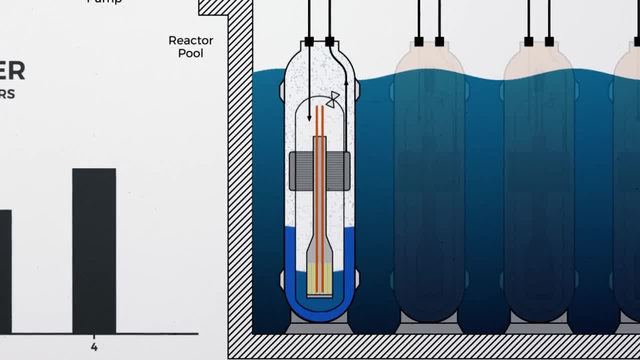 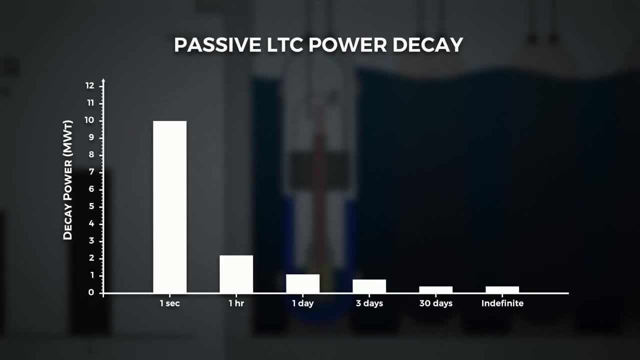 bottom of the reactor vessel, creating a natural circulation of cooling water inside the steel containment vessel. Within seconds the energy and temperature drop drastically and within a day the thermal power drops by 90%, cooling off the last 10% over the course of weeks. 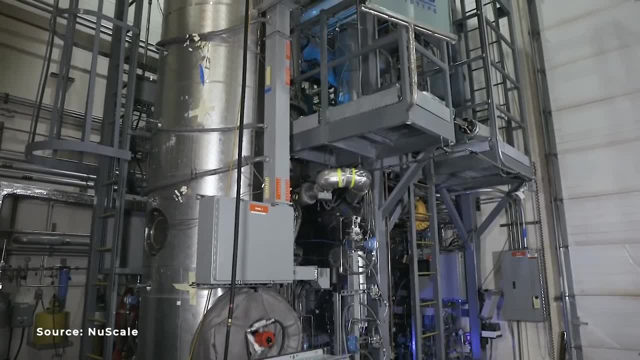 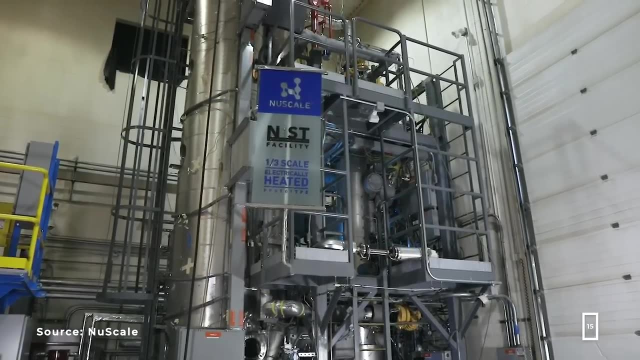 And while this all sounds great, We are nowhere near commercial deployment. NuScale is by far the most ahead, but have only managed to create a 1 third scale model of their power plant. Other countries like Russia, China, France and South Korea have also invested in creating 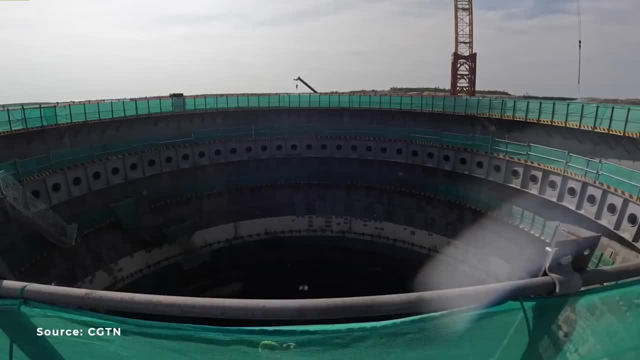 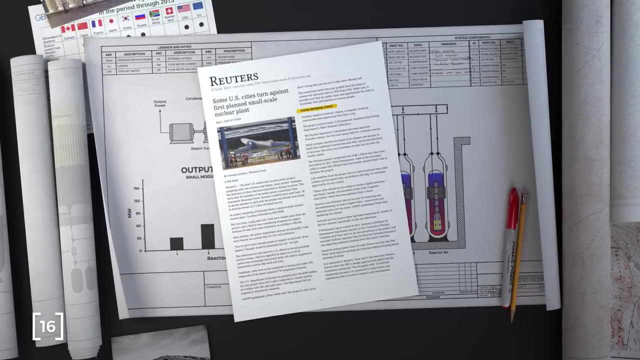 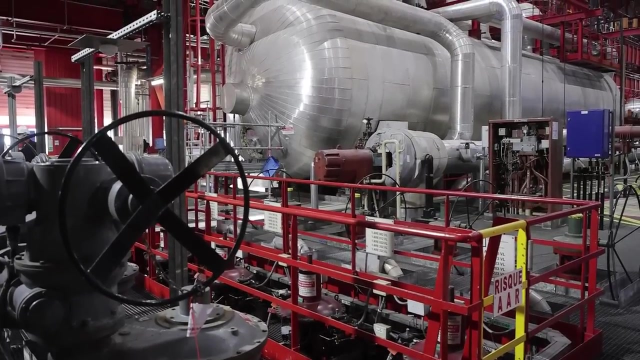 SMR technologies, but have struggled to find utility customers. Without potential customers, these start-ups will always fail in a capitalist system. Even NuScale has been dropped by some utility clients as their prices seem to have exceeded expectations. This poses a massive challenge to companies that rely on large scale standardised factories. 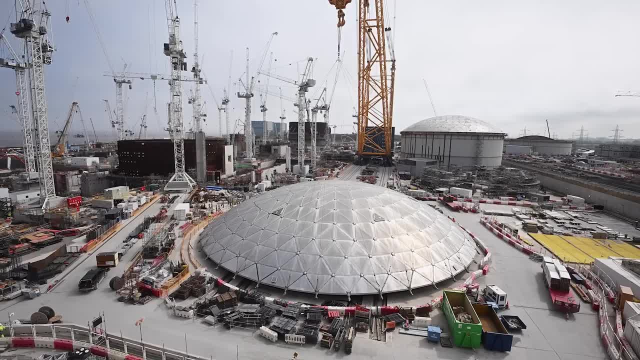 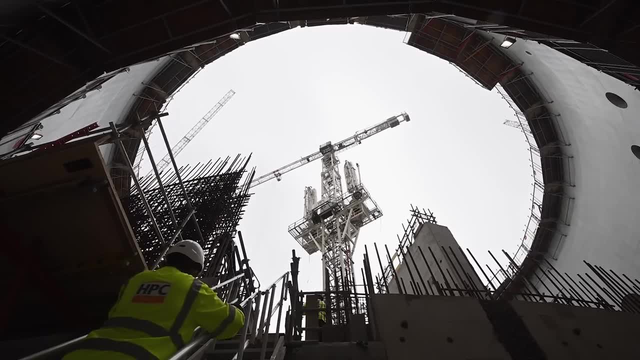 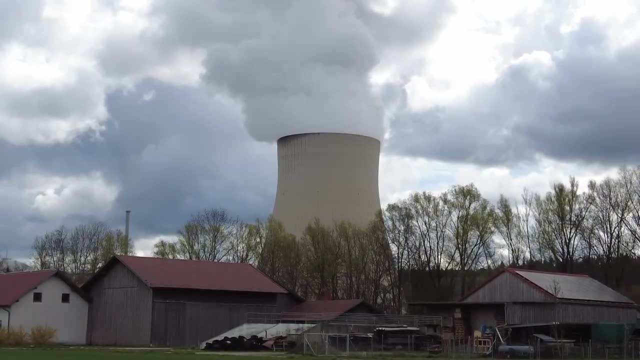 to achieve their key market advantage. To build the factory they need customers, but they can't get customers without the factory. Thousands of reactors will need to be built before economies of scale can kick in and, in reality, the exact reason traditional nuclear reactors produce so much electricity is to 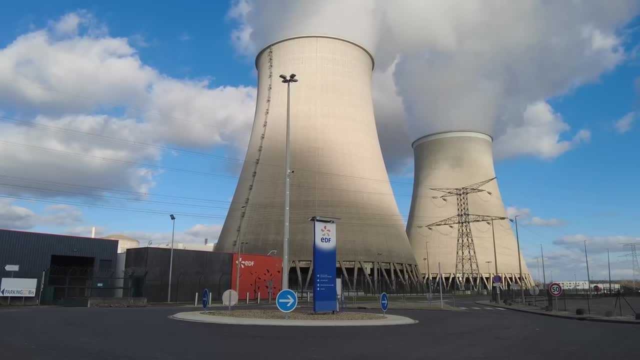 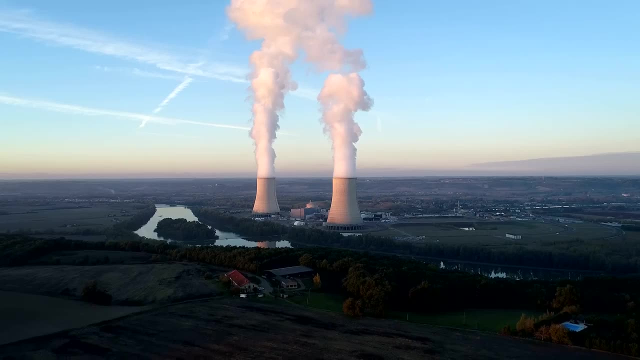 benefit from the economies of scale. Building a 1,000 megawatt reactor reduces the cost. The cost of building a 1,000 megawatt reactor reduces the cost of building a 1,000 megawatt reactor And that's the most important metric in the electricity market. 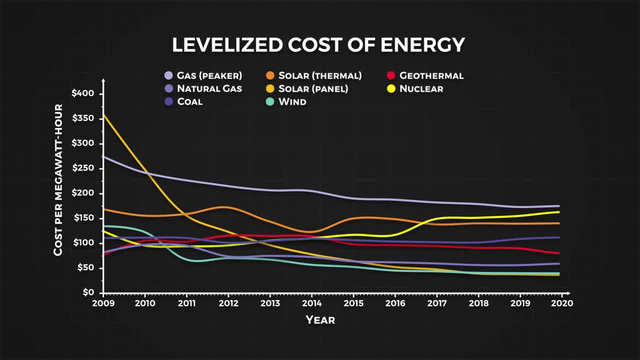 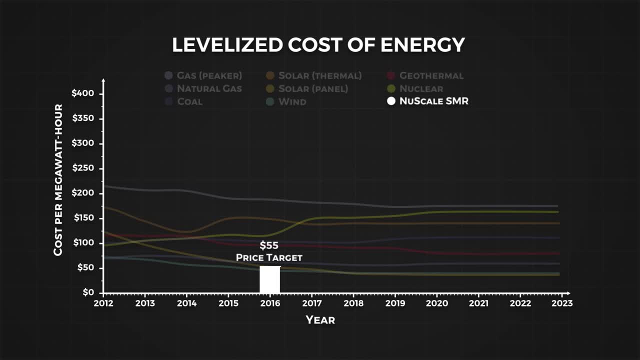 That's how you get grid operators to buy your electricity: by making it cheaper. NuScale's original price point was $55 per megawatt hour. However, due to inflation, rising steel costs, development issues and many delays, the costs are now estimated at $100 per megawatt hour. 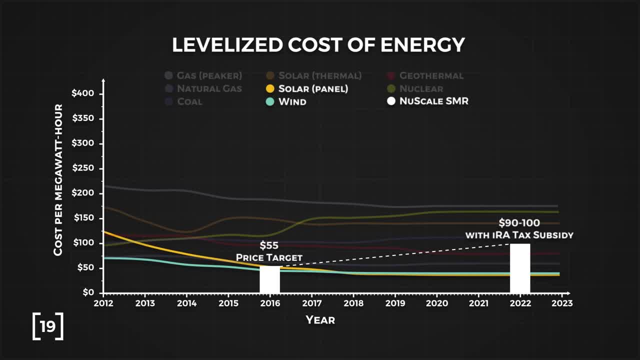 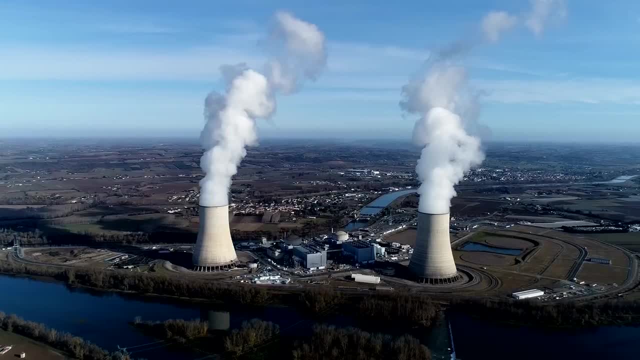 In comparison, onshore wind and solar can be as cheap as $30 per megawatt hour. With the threat of climate change looming over us, we need to ask ourselves: can we rely on a capitalist system to fix a problem driven by capitalism? There is a distinct possibility that these technologies will never succeed without government funding. Energy generation is the foundation of every major world economy, and it is in countries best interest to invest in these technologies. Nuclear energy provides energy security. The US is not the only country in the world to invest in these technologies. 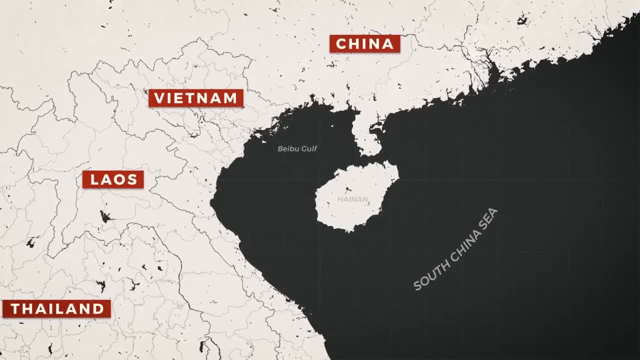 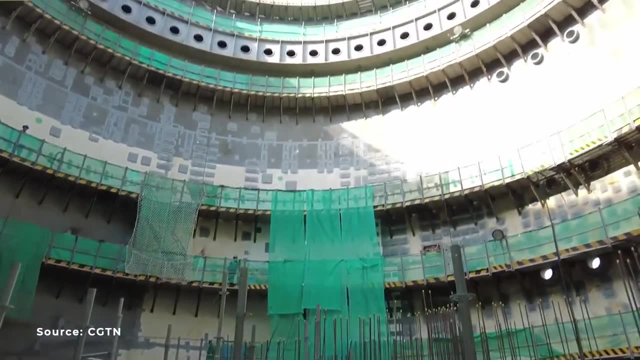 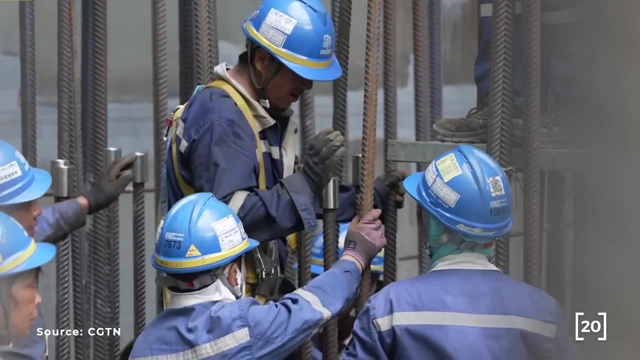 China is not alone in trying to develop the technology. China has embarked on the construction of a functional small modular reactor project. here, However, similar to many nuclear ventures, costs have significantly escalated, with the SMR reportedly being twice as expensive in terms of cost per kilowatt hour compared to. 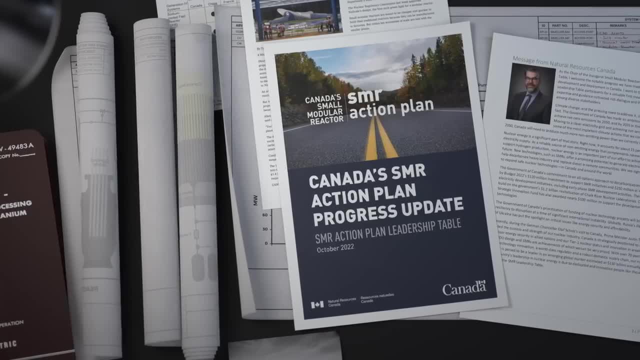 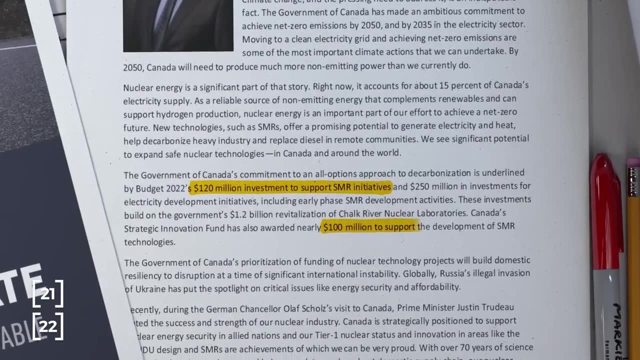 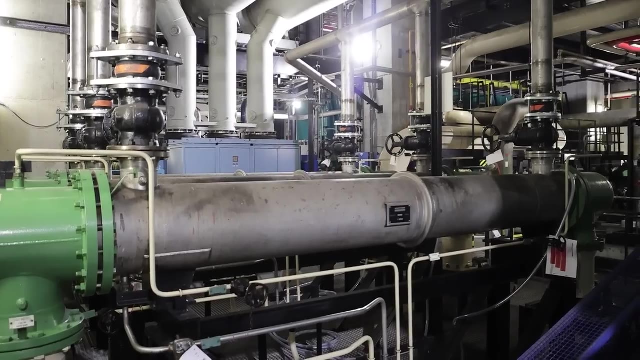 a traditional large scale nuclear plant. Canada has formulated a 2020 SMR action plan to help bring down costs and have invested millions of dollars in the project. The goal is to bring the dollars into SMR startups Developing these technologies will need vastly more money than this, but it's a step in. 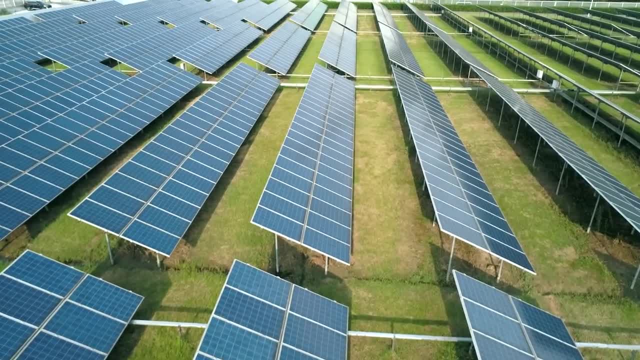 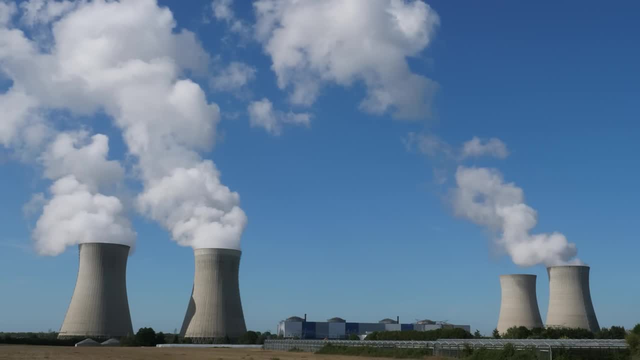 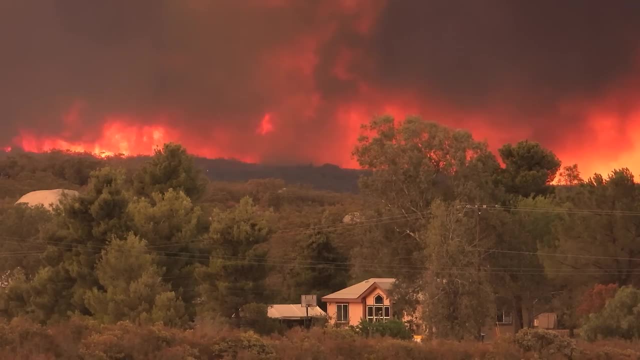 the right direction. Wind and solar are game changing technologies that we could only have dreamed of being as cheap as they are today two decades ago. But we need every tool at our disposal to fight climate change, Not just to decarbonise our energy generation, but to start fighting the effects of climate. 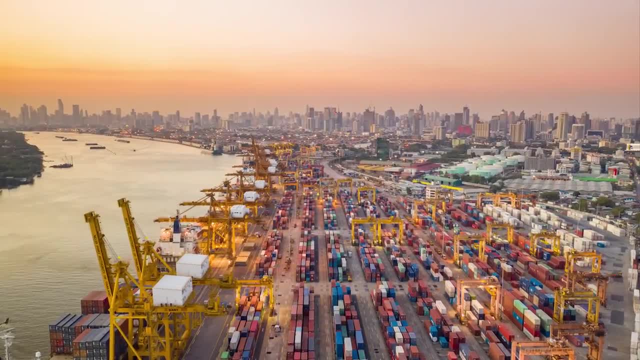 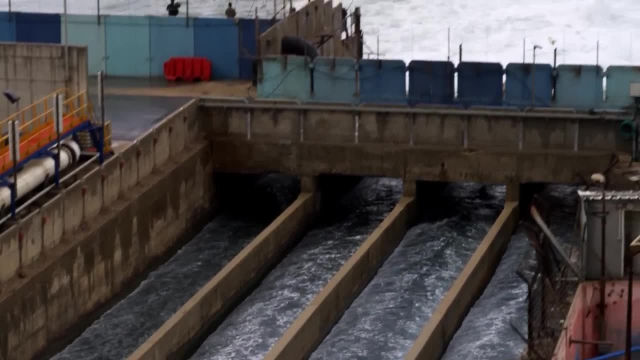 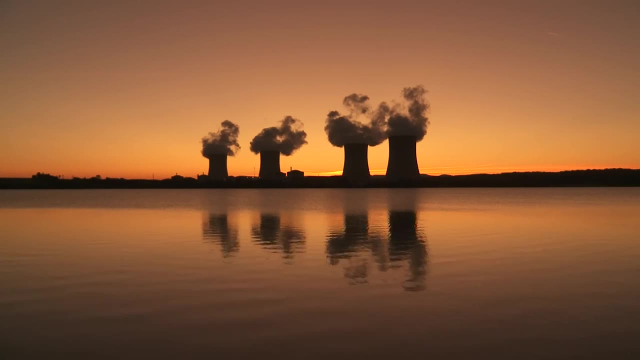 change, population growth and global industrialisation. From increasing demand for air conditioning, water scarcity driving the need for energy intensive water desalination, to last ditch efforts to reverse climate change with carbon capture, Energy is the cause and solution to our problems. 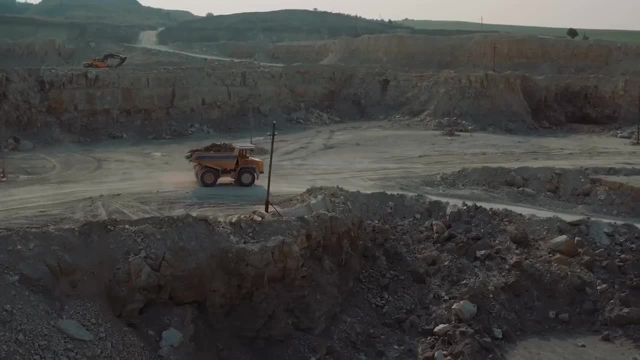 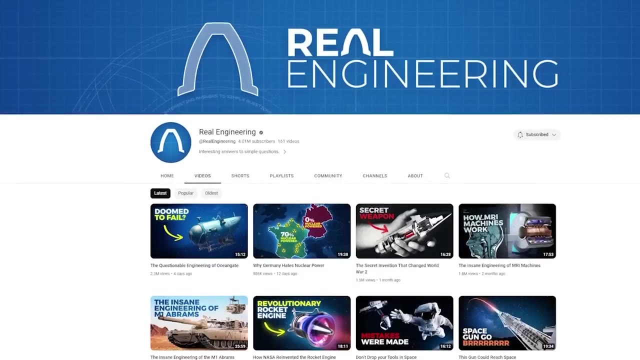 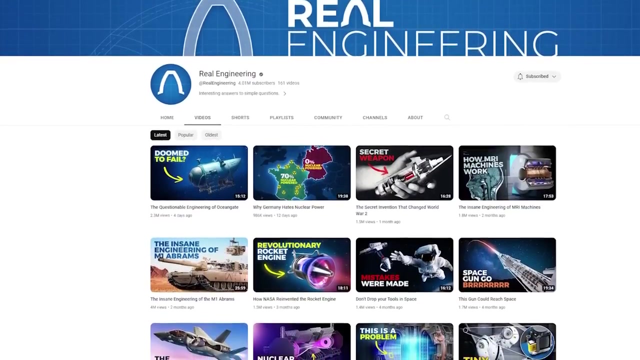 The transition from fossil fuels, in my opinion, is the most pressing issue facing humanity. This is an all hands on deck problem. We need our best minds working on it, and I see it as part of my responsibility, with a platform as large as mine, to inspire the next generation of engineers to work on the